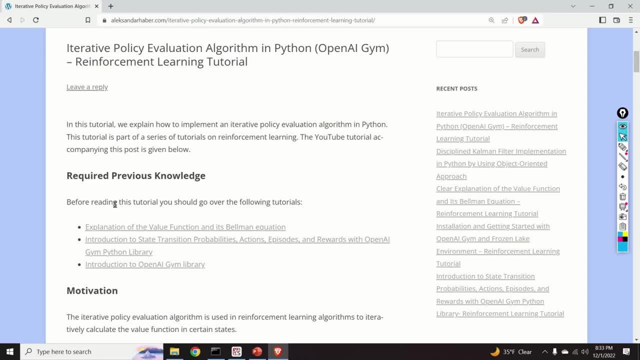 Hello everyone and welcome to Reinforcement Learning Tutorials. In this tutorial, I will explain you an Iterative Policy Evaluation Algorithm. I will explain you how to implement this algorithm in Python and at the end of this video, we will test the performance of the Iterative Policy Evaluation Algorithm in the Frozen Lake environment from the Open. 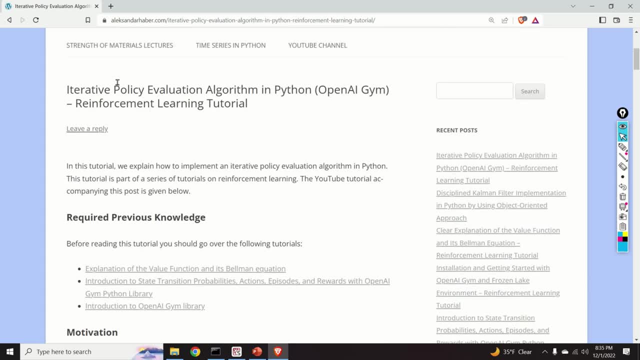 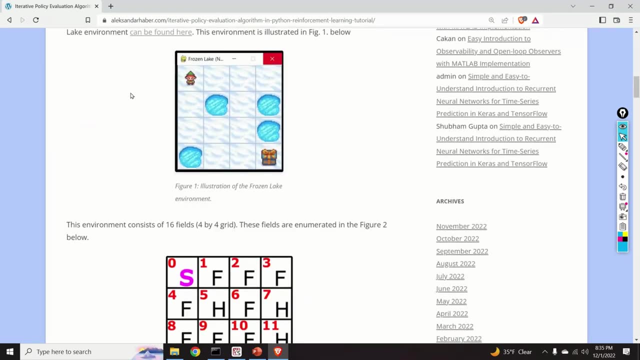 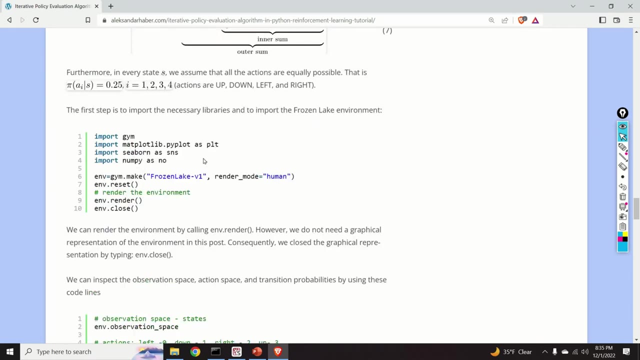 AI Gym. As always, I created a post that nicely summarizes everything that I will explain in this video. This post contains all the explanations, graphs, and it even contains Python codes that you can see over here. A link to this post is given in the description. 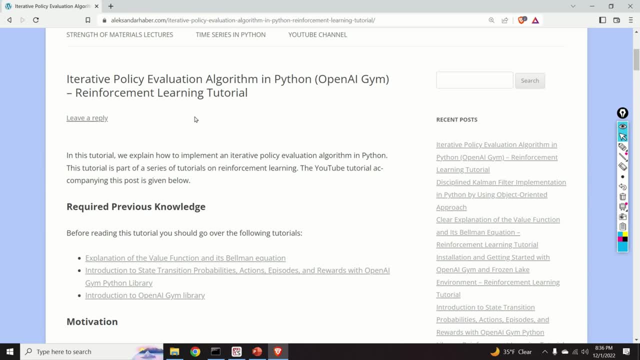 below And before I start, I would like to mention the following: It took me a significant amount of time, energy and planning to create this video. I would like to thank you for watching this video and this post. Consequently, I kindly ask you to press the like and subscribe. 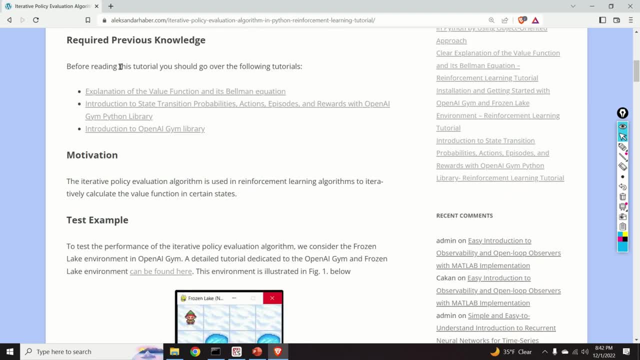 buttons. Thank you very much. Ok, so let's start with the required previous knowledge Before watching this video tutorial. it's a good idea, and I strongly suggest you, to go over the following topics. First of all, you need to become familiar with the value function and its Bellman equation. 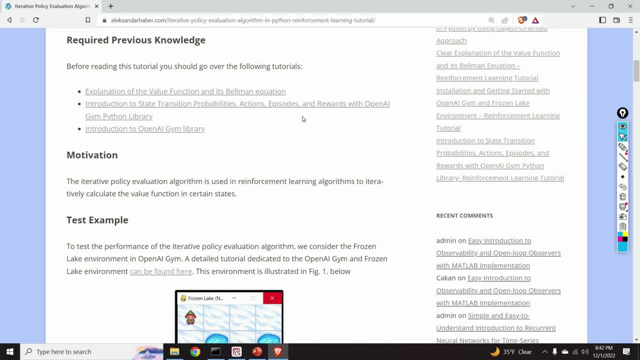 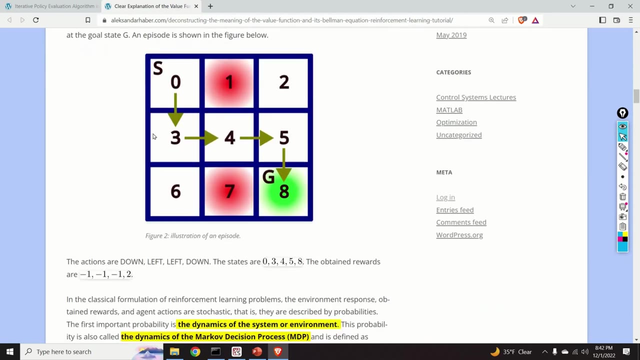 Luckily, I created a post and even a YouTube tutorial that summarizes these important topics. So you can click over here, you can follow the link and you can read this post that summarizes the value function and that explains the Bellman equation. Then you need. 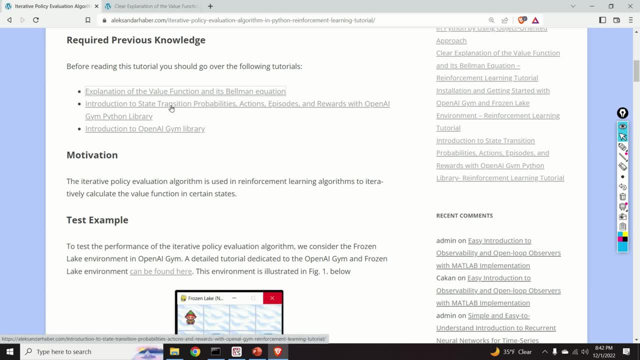 to become familiar with state transition probabilities, actions, episodes, rewards and the following words, And you need to become familiar with the Open AI Gym library. You can learn these topics by following the second link And here's the post. And here are two YouTube. 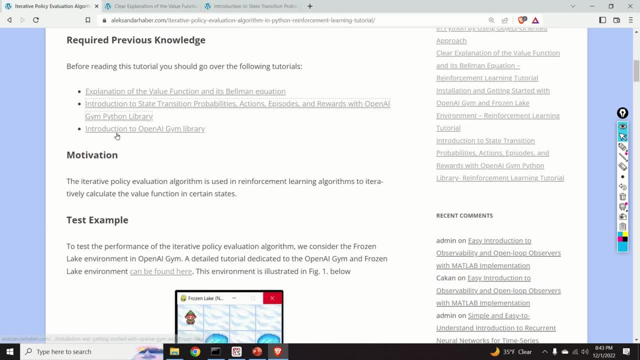 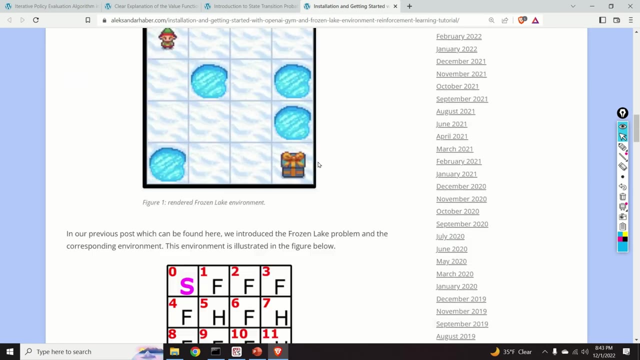 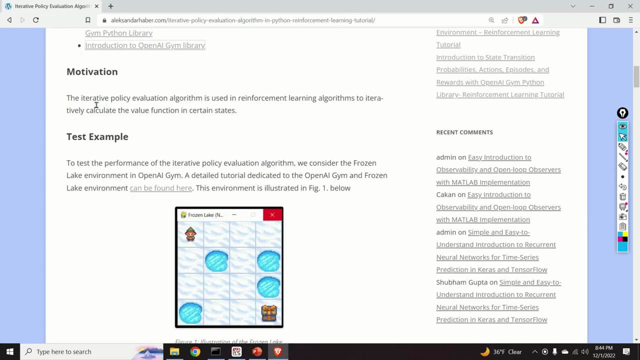 video tutorials. Then you need to become familiar and to gain experience in using the Open AI Gym library. And again, you can click on this link And read the post that will teach you how to use the Open AI Gym library. Ok, under the assumption that you obtained enough background information and background. 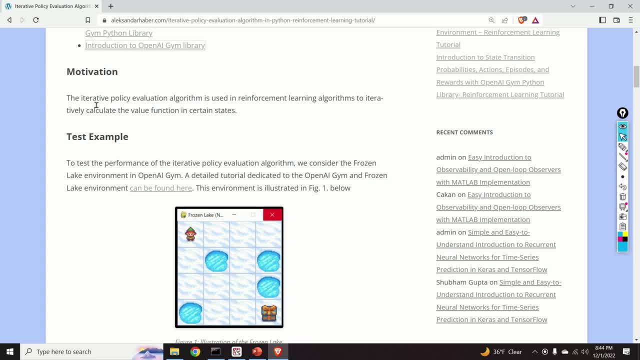 knowledge. we can continue with this YouTube tutorial, So let's start with the motivation. The iterative policy evaluation algorithm is used in reinforcement learning algorithms to calculate the value function at certain states. Then let us repeat this motivation once more, since it's very important from the beginning. 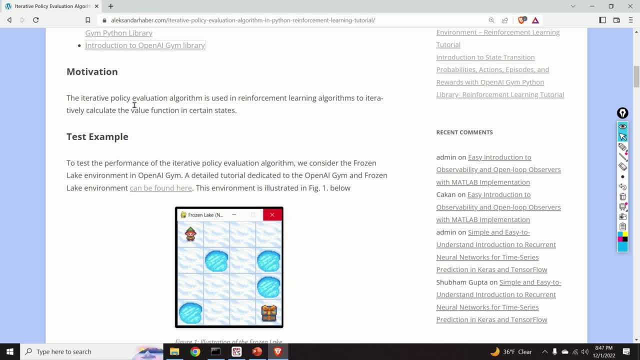 of this video that you get the main points. After the first video, let's go through a few rules For a given policy. the iterative policy evaluation algorithm is used to iteratively calculate the value function at a given point. In addition, we can factor the solution for the creating of the evaluation model in place. 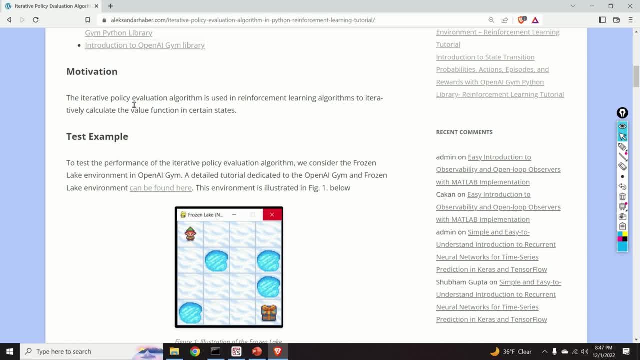 of it. Now, the iterative policy evaluation algorithm should be used under this objective Between different columns of the burden-free. accordingly, the prioritization of this automatic evaluation algorithm is a competition of having the initial Нам to this maximum value, certain states and this algorithm is a building block of more complex 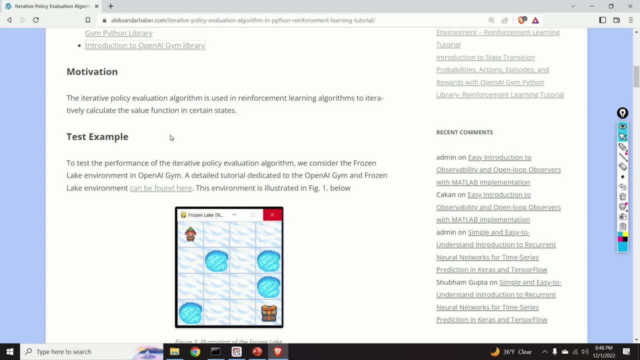 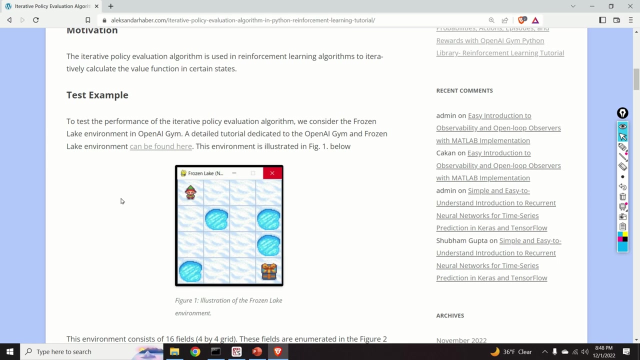 reinforcement learning algorithms. that's why it's very important to completely understand all the ingredients of this algorithm. so let us immediately jump on a test example in order to make this video more interesting. to test the performance of the iterative policy evaluation algorithm, we consider the frozen lake environment in open AI gym, a detailed tutorial dedicated to the open. 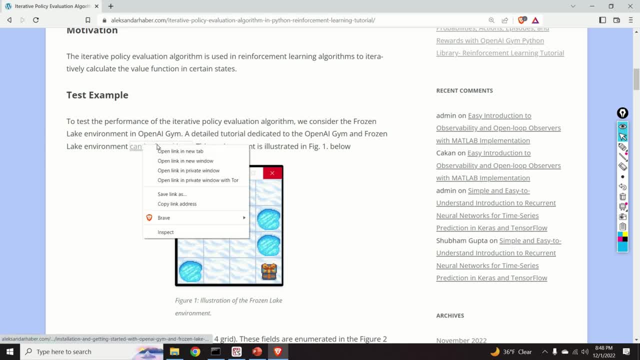 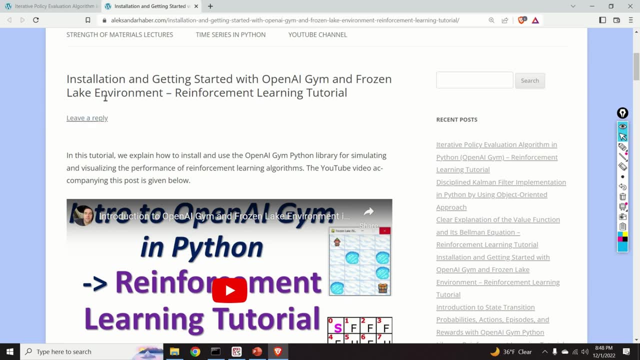 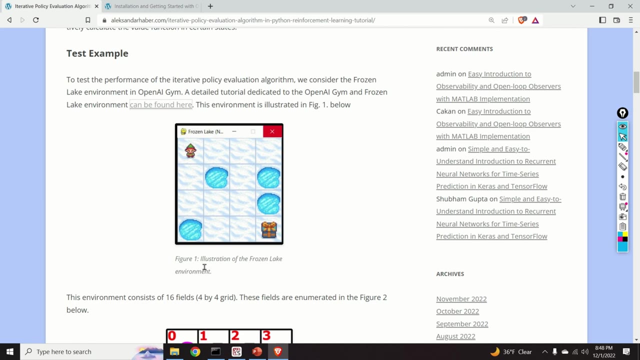 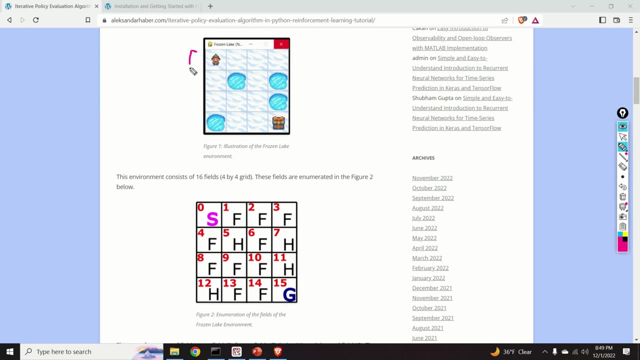 AI gym and frozen lake environment is given over here. you can follow this link to learn more about the open AI gym and the frozen lake environment. this environment is illustrated in the this figure. the frozen lake environment consists of 16 fields, that is, we have a grid of 4x4. to every field we associate a number. here is the number 0. this is 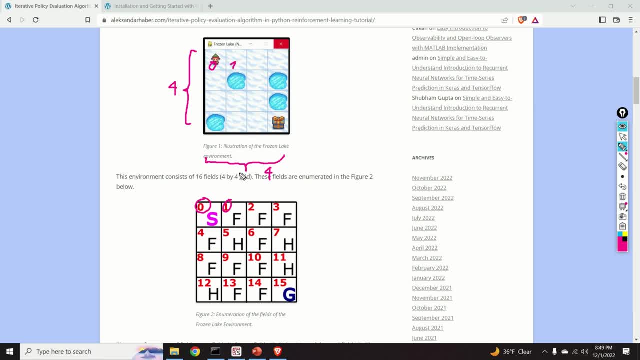 the field 0, here is the field number one, here is the field number two and the final field is the field 15, that is the field given over here. then there are four types of fields. the first type is the start field, here or over here. then we have frozen. 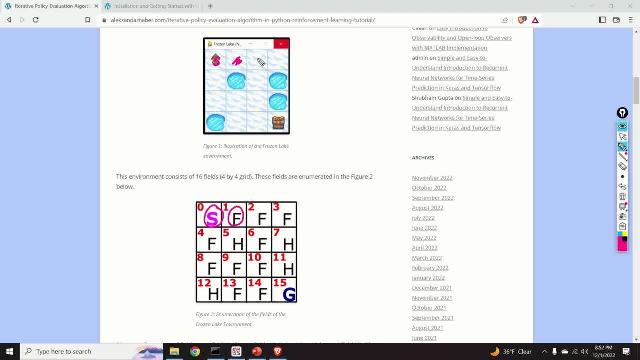 fields F, here the frozen fields, then we have holes, here the holes, and finally we have the goal field over here, or sketched over here. the goal of the game is to reach the goal field G, starting from the start field s and by avoiding the whole fields. for example, a successful game can look. 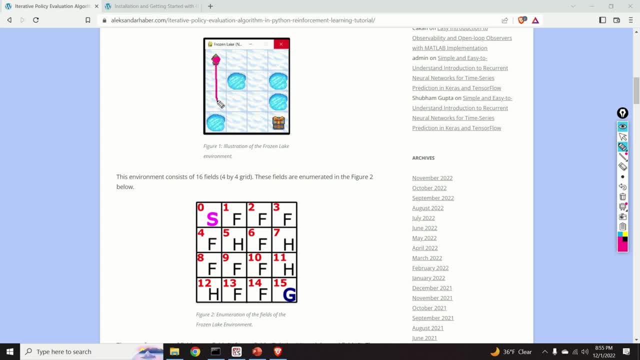 like this: we start from here, we go down, then we turn right, then again we go down and we reach our destination or our goal field. here it should be kept in mind that if you're at the frozen field, for example over here, we can only move left, right, up or down. we cannot move. 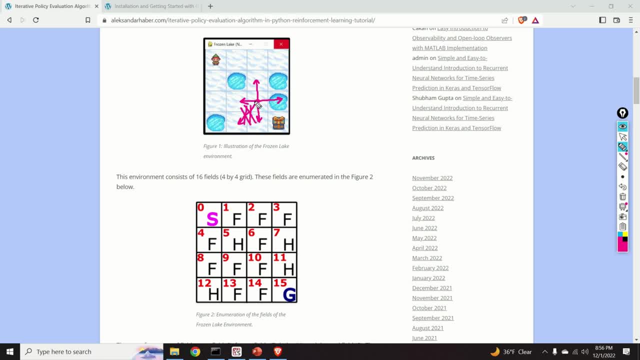 diagonally. so this movement is not allowed or this movement is not allowed, the game ends unsuccessfully if we step on the whole field. for example, if you start our game from here, we go right and then we go down and we step on the whole field, we end our game unsuccessfully. 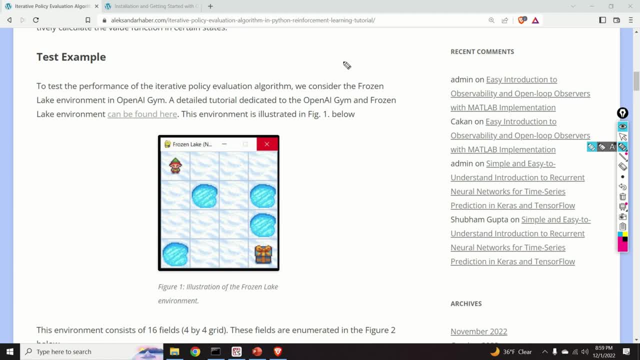 and finally, let's talk about rewards, since reinforcement learning is all about rewards. if we step on the frozen field, that is, we step over here, we get the reward of zero. similarly, if we step on the whole field, we also get the reward of zero. and if we step on the goal field, we get the same reward over here, the correct. 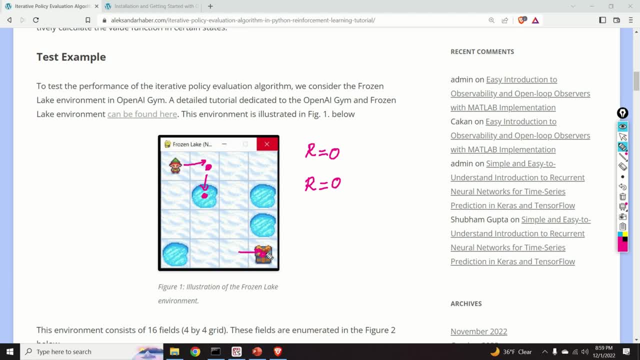 religious reward, the whole field, the old field. we also get the reward of zero. on the field zero and on the periferical combat field we got the reward of five in a result of the, That is, if we end our game successfully, we get the reward of 1.. 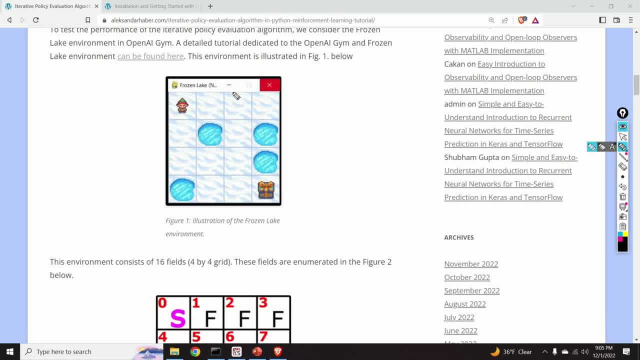 With every field we can associate a state. For example, with this field, we can associate state S1.. With this field, we can associate state S2.. With this field, S3.. With this field, S4.. And finally, with this field, S16.. 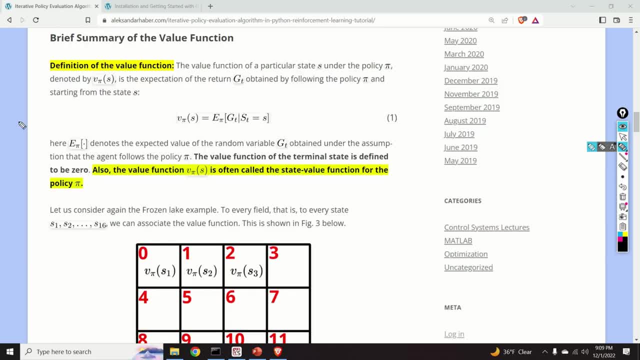 After introducing the frozen lake example, we are ready to briefly summarize the value function and to relate the value function with the frozen lake example. So what is a value function? The value function of a particular state, S under the policy pi denoted by V in the index pi of S. 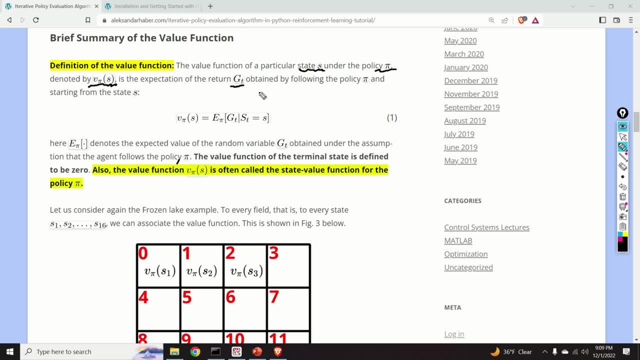 is the expectation of the return G. Gt obtained by following the policy pi and starting from the state S. Here is the equation that defines the value function. Gt is the return. You can think of the return as the sum of the rewards. 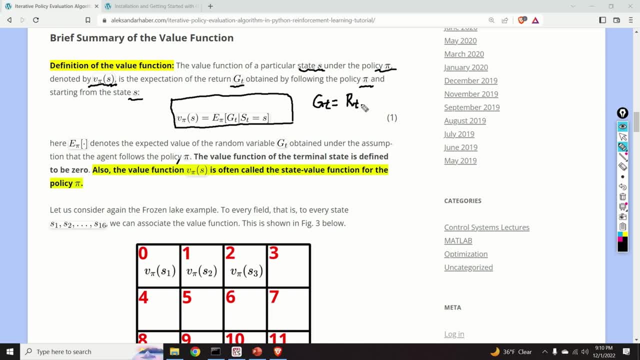 starting from Rt plus 1 plus Rt plus 2 and until the end of the episode or until the end of the game, where Rt plus 1 is the reward obtained at the state St plus 1, Rt plus 2 is the reward obtained at the state St plus 2,, etc. 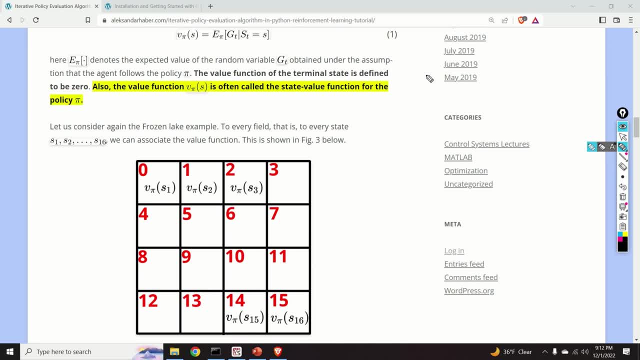 Here it should be kept in mind that the value function of the terminal state is defined by the value function of the terminal state. It is defined to be 0.. So what are the terminal states? Going back to our example, that is, to our frozen lake, 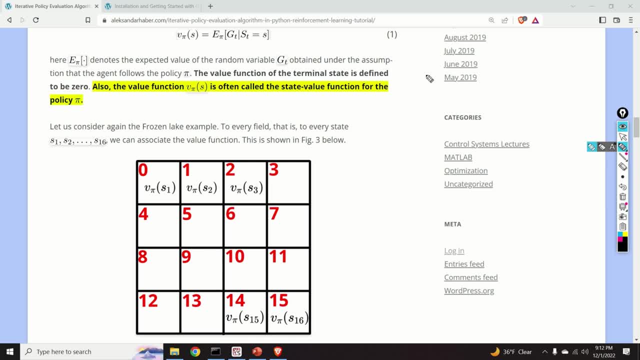 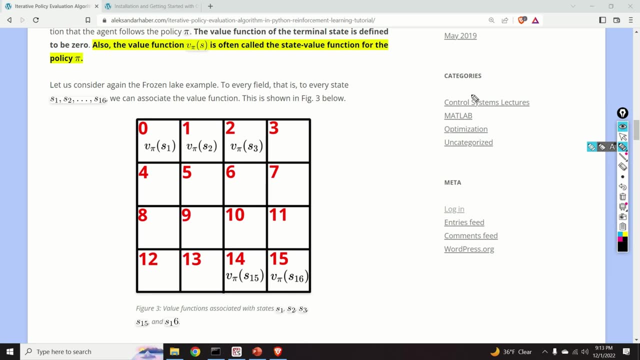 the terminal states are the states that terminate the game, And these states are obviously the whole states and the finer or the goal state. Let us go back to the frozen lake example, To every field, that is, to every state, S1,, S2,. 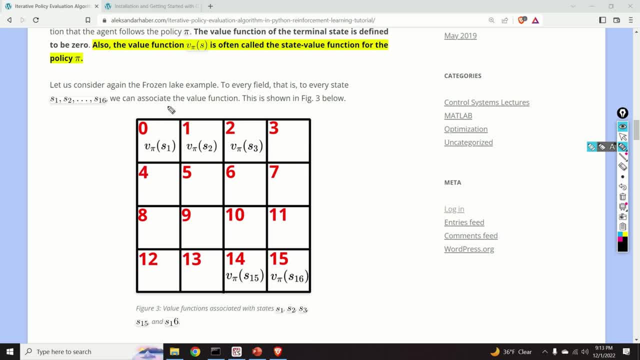 until S16, we can associate the corresponding value function. Here is the value function of the state S1.. Here is the value function of the state S2.. Here is the value function of the state S3.. Similarly, here is the value function of the state S16. 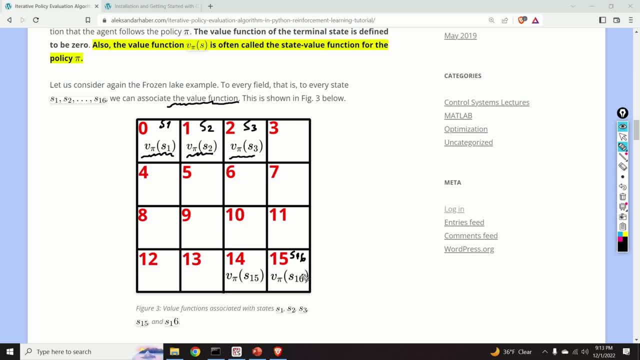 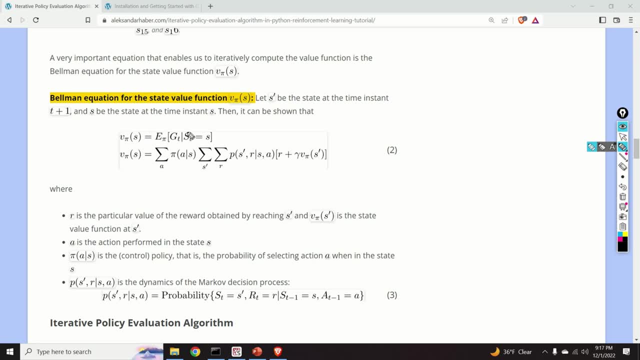 and the state S16 is the goal state. A very important rule in this level is that every domain should have a value function and every state should be defined by an even number, A very important equation that enables us to iteratively compute the value function. 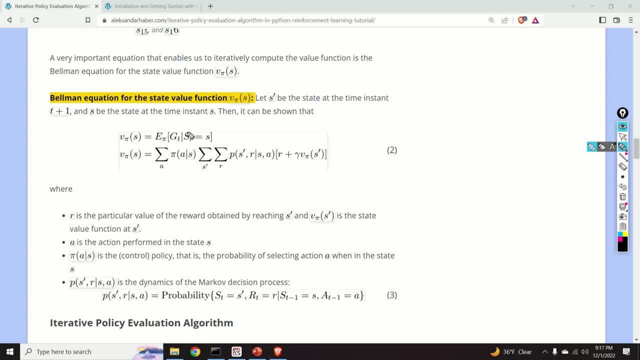 is the Bellman equation. The Bellman equation is given by the equation number 2.. Let us briefly explain the true meaning of the Bellman equation And let us consider our frozen lake example. Let us assume that we are in the central field. 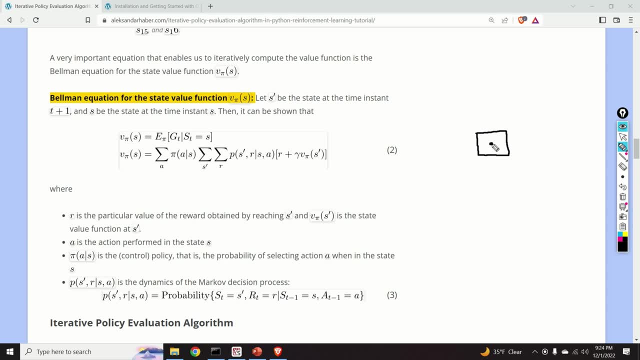 That is, that we are in this field, And let this field, or better to say, its state, be denoted by S. Then let us assume that we are following the policy pi selecting A, given that we are in the state S. 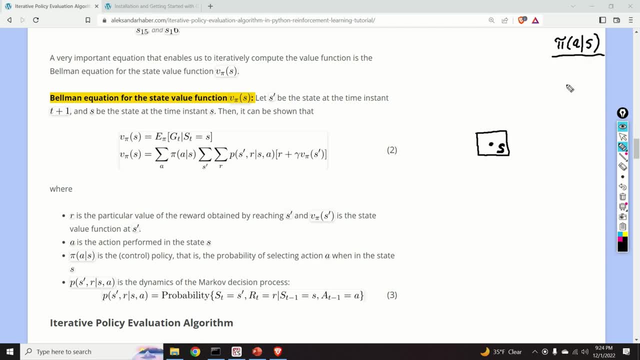 So this is actually a probability of the state S. So this is actually a probability of the state S, So this is actually a probability of choosing a particular action. A given that we are in the state S, We have four possible actions. 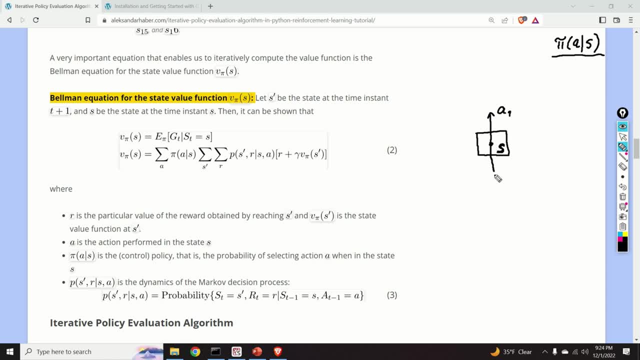 We have action A1 going up, action A2 going down, action A3 going left and the action A4 going right. This graph corresponds to the sum over here, So the summation is performed over A1,, A2,, A3, and A4.. 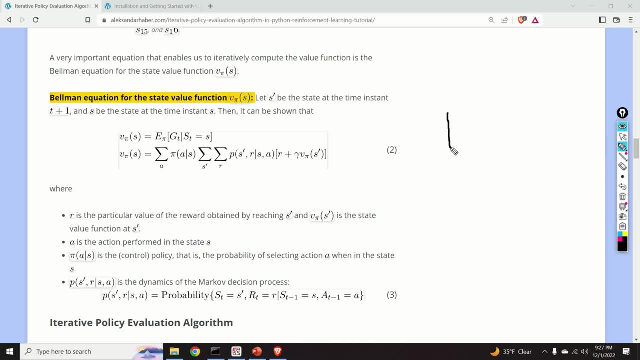 Next, let us assume that we are in the state S and that we selected the action A1,, A2,, A3, and A4.. Next, let us assume that we are in the state S and that we selected the action A1, A3, and A4. 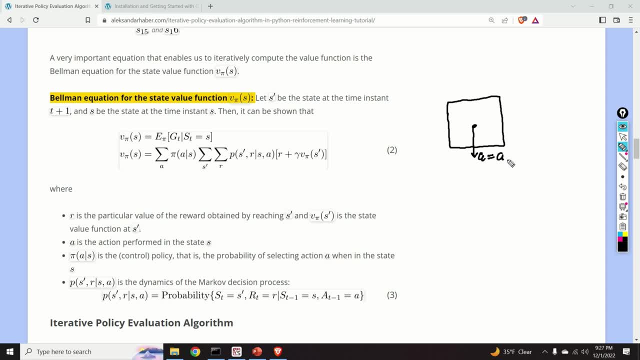 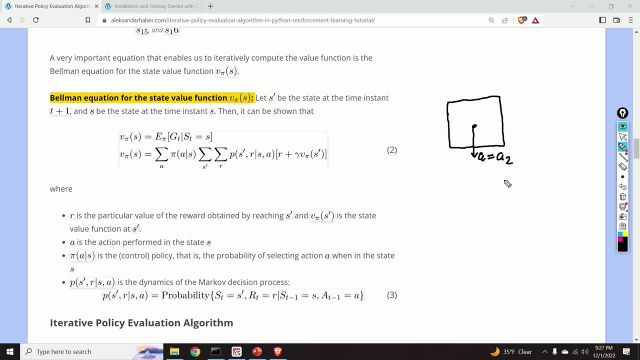 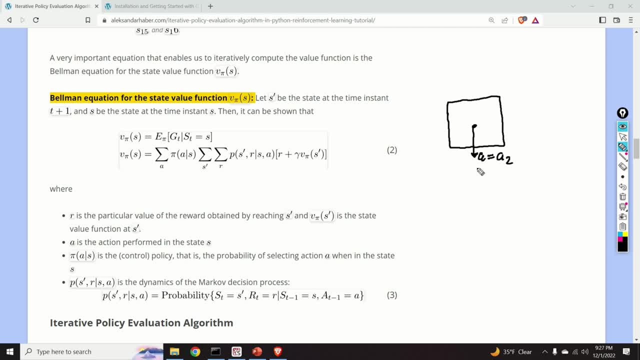 Next, let us assume that we are in the state S and that we selected the action A1,, A3, and A4.. Next, let us assume that we are in the state S, completely probabilistic, or better to say, stochastic, even if we're in the state s and we 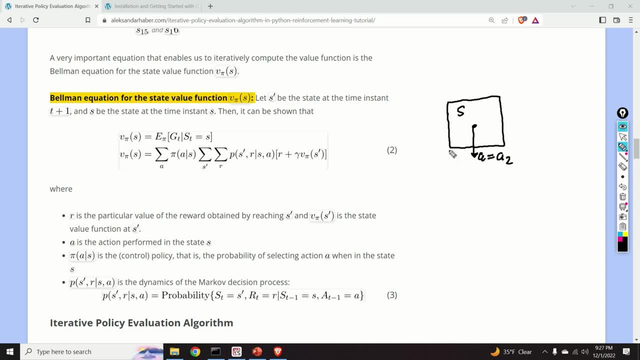 selected the action a2, that doesn't mean that we will necessarily go to this state, that is, to the below state. since this is a frozen lake, the floor is very slippery. if we want to go down, it might happen that we in reality can go left or right. that is, there is a certain probability. 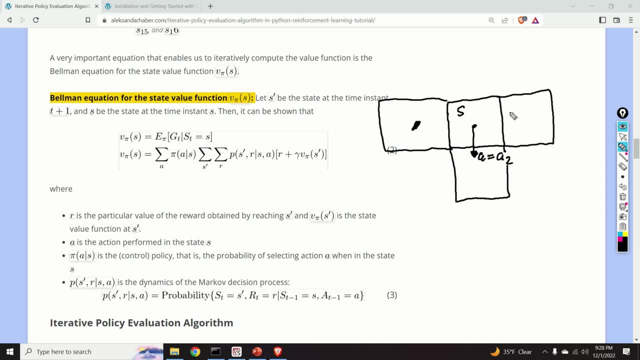 of going to this field or to this field, if we selected the action go down, of course, there is a certain probability of going to our intended destination, or there is a certain probability of even going down upwards. these probabilities are encapsulated or governed by this probability that's called the. 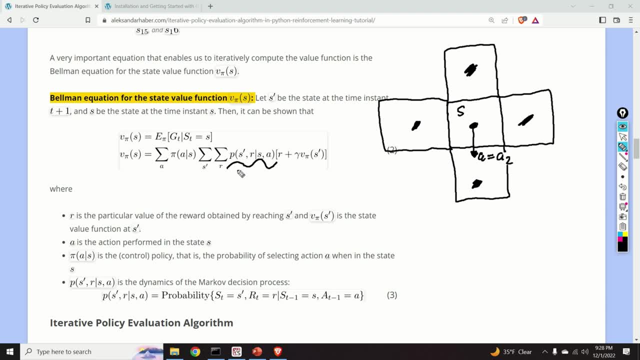 dynamics of the mark of decision process. again, probability pi- given that that we are in the state s and that we selected the action, a is the probability of going to this field or to this danger state, then this probability can be a good signals. but this will be of. 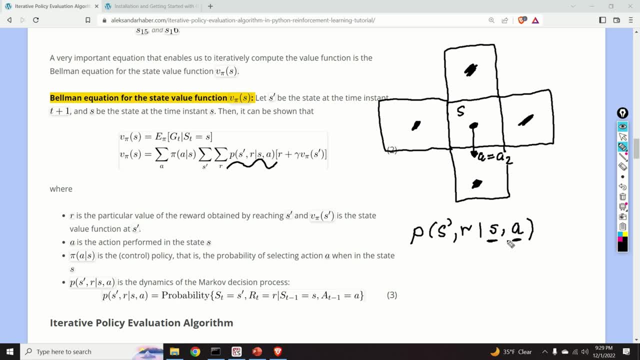 actually being just the suggests that we cannot even go down the slope poor at this point because this 온 is a non free state. so this probability we are actually going to be normal instead of up to our ultimate destination point. so this can be s' and this one as prime, for example, to this particular state in terms of spicy raze. 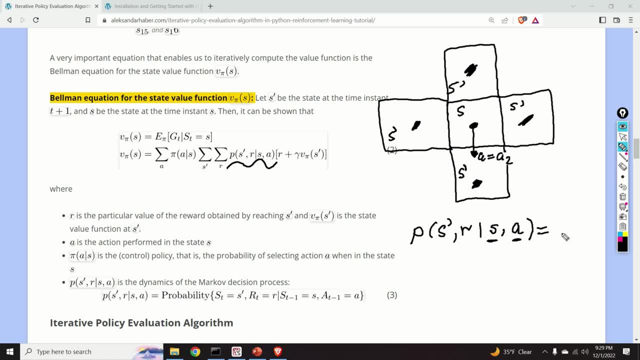 case, we can assign this probability to be equal for all of these S' let's call this S'1,, let's call this S'2,, S'3 and S'4.. So the probability of reaching of any of these states- S1', S2', S3' and S4' given that we are in the state S and that we have selected, 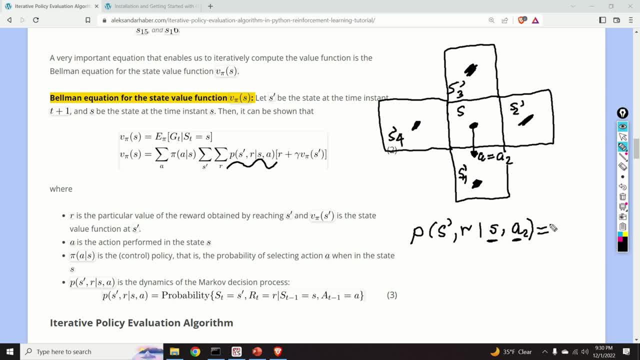 a particular action, Let's say the action A2, can be, for example, 0.25 or 1 over 4.. So there might be an equal chance of going to any of these fields. if we were in this field and if we selected the action GO DOWN, Then by reaching the particular 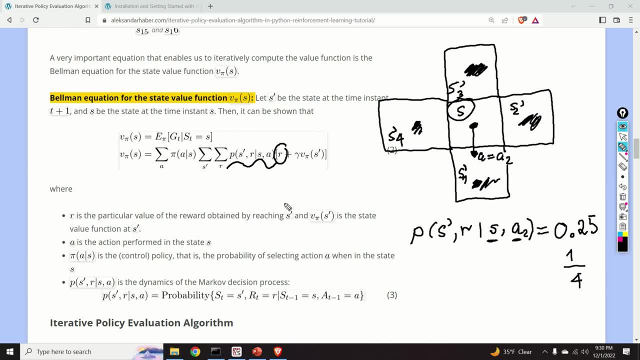 A2, state s prime, you obtain a certain reward, denoted by R, and we have a certain value function at that destination state, and this value function is denoted by V PI of s prime. and finally, we are ready to give a summary of the Bellman equation. for that purpose, let us consider the frozen. 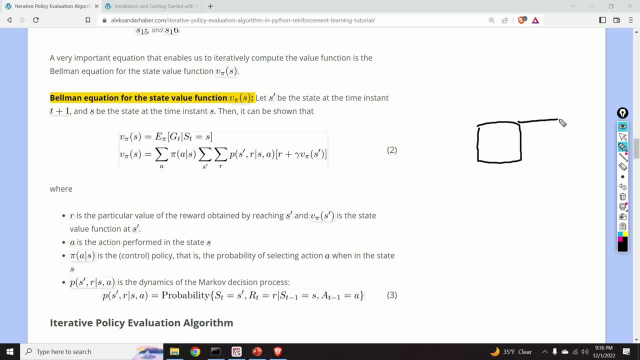 lake environment. this is our central field. and let us consider the four neighboring fields. the current state is this state s, and we have four possible next states. these states are s 1 prime, s 2 prime, s 3 prime and s 4 prime. to every next state we can associate a value function, so this is value function. 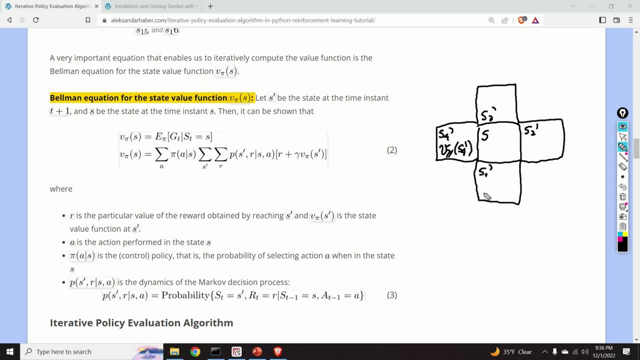 at s 4 prime. this is the value function at s 1 prime, this is the value function at s 2 prime and this is the value function at s 3 prime. the Bellman equation enables us to compute the value function for this central field, or for the current state, on the basis of the value functions defined for. 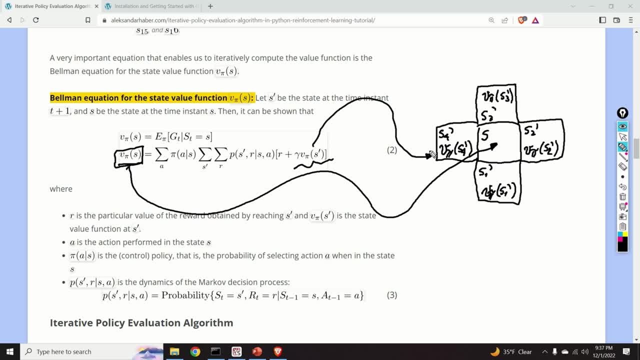 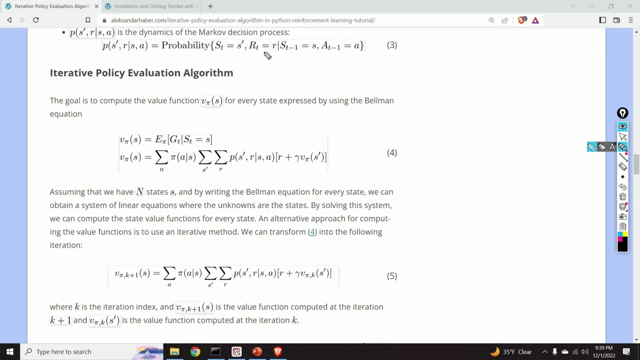 all possible future states and on the basis of the reward obtained by going to the future state, and on the basis of the transition probability or the basis of dynamics, and on the basis of the policy. now we are ready to explain the iterative policy evaluation algorithm. the goal of this algorithm is to compute the value function of this. state by one day. so this is the right expression, so the error should be accurate. once we have been Kivolowitz's, we compute the value function of this step by step. здоров, no, in several cases besides this, the martian line in the expectation of the 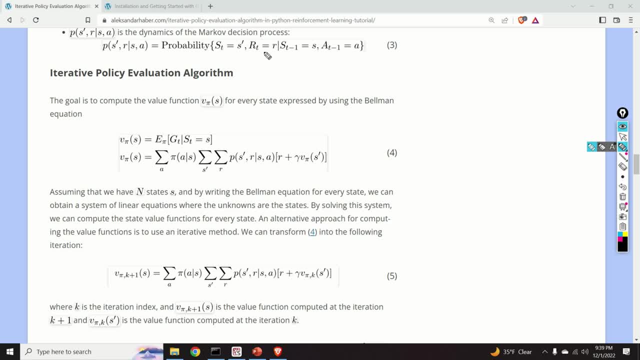 layer. she will be arriving first on board with a marketers. so we become the friends of the, the squareelen. right here on the a n Idl, which is theells, we take tohyun value function for every state, and this value function is expressed by using the. 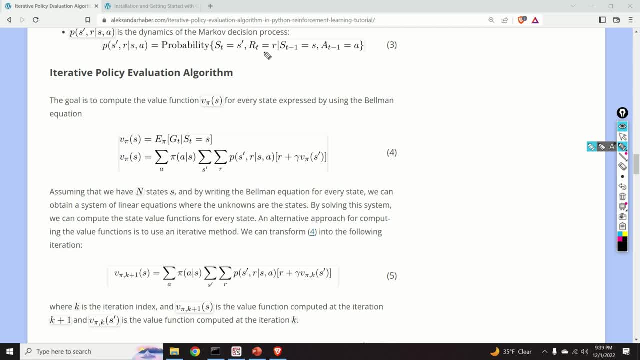 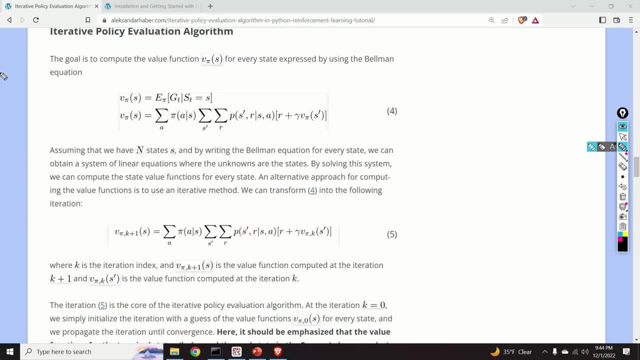 Bellman equation, or better to say, we use the Bellman equation to compute the value function. let us assume that we have n states- s1, s2, s3 until SN. for every state we can write the corresponding Bellman equation. for example, for the state s1 we can write value function pi at the state s1 is equal to the right. 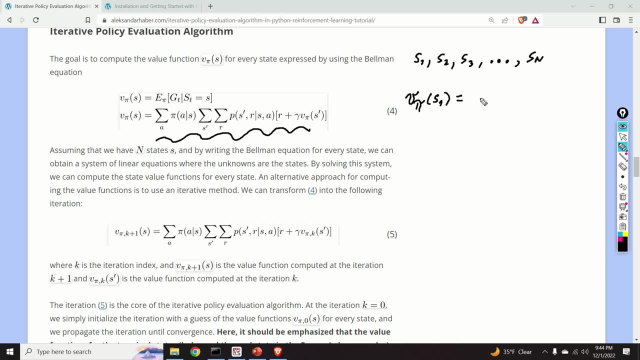 hand side and for simplicity I'm not going to write the right hand side. it's important to note that the right hand side will be again a function of the value function. then we can write the value function for the state s2 and we can use the. 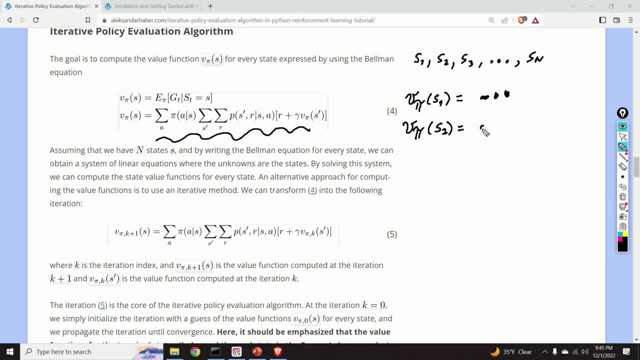 Bellman equation to express the right hand side. again here I will write three dots. by repeating this process we will end at the value function at the state SN, and again we can use the Bellman equation for the state ofossa. so here we're: verschiedene N, double sets of N. 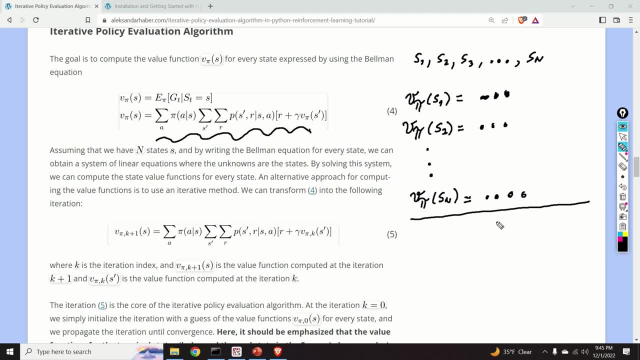 variable and nanometer can express the saying that, since I have a between N and the paralleleted result, I can express the right hand side. we can now examine some equations to solve the problem. so let's solve an unknowable value function plus the value function, the value function ofwhat we chose in. 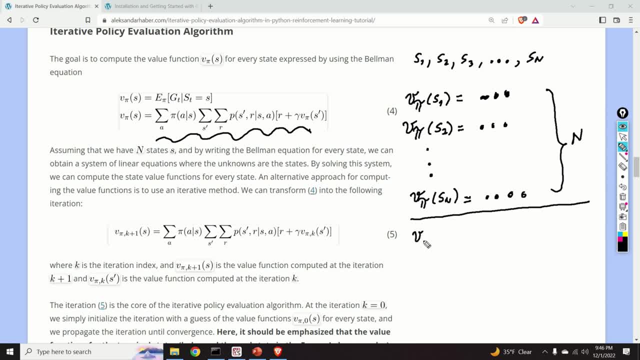 the weekpoint number of elements. and let us analyze these equations. we have a system. we can: s1,, then v pi of s2, three dots until v pi of sn, Under the assumption that the transition probabilities or that the dynamics of the system is known, and under the assumption 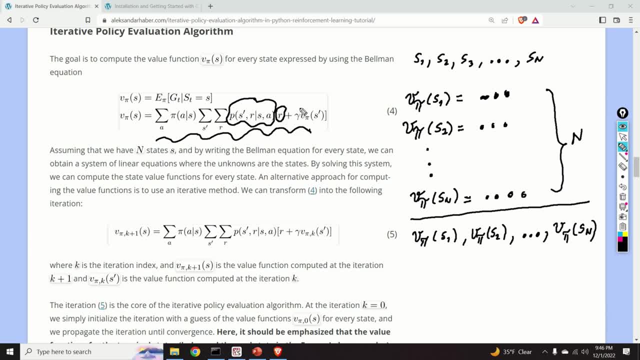 that the reward values are known and under the assumption that this coefficient is known and under the assumption that the policy is known, we obtain a system of n equations with n unknowns And since this is a linear system, under mild assumptions we can solve this. 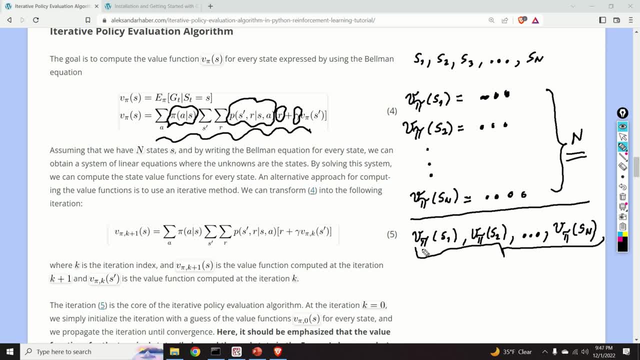 system and we can compute the value functions at the states s1,, s2, until sn. This was one approach for solving this system. However, there is another approach that, in my opinion, is more elegant, And this approach relies upon an iterative. 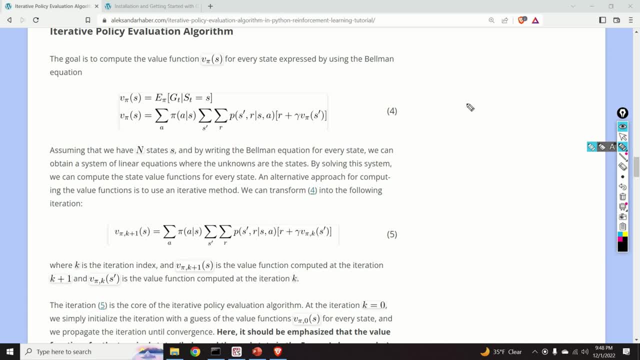 solution. So what is the idea? In order to explain the main idea, let us consider a fixed point iteration. Let us assume that we want to solve the following non-linear equation: x is equal to f of x, where f is a non-linear function. How to solve this equation? Of course we can. for example: 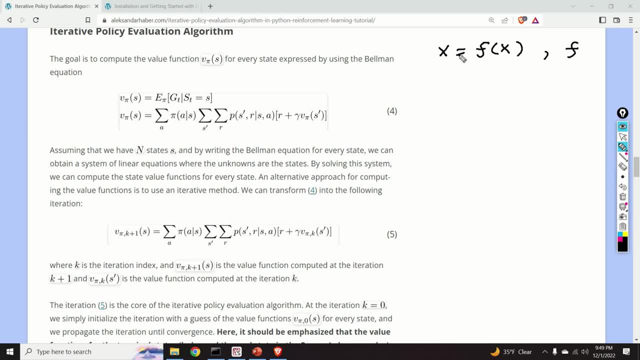 use Newton's method. However, is there a more elegant and more numerically tractable way for solving this equation? Of course There is such an approach. Under some mild assumption, we can define the following iteration: xk plus 1 is equal to f of xk. 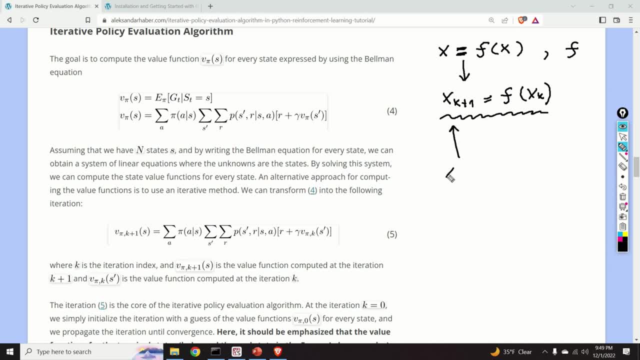 By initializing this iteration with some x0, and by propagating this iteration, the value of xk, when k goes to infinity, will approach to our true solution. That's denoted by x star. Again, here is the idea. We start the iteration with x0. And we compute. 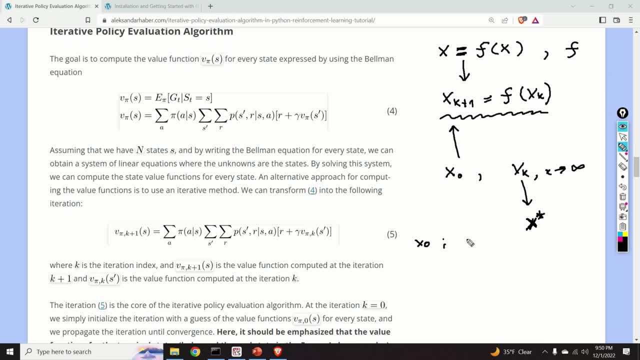 x1, simply as f of x0. Then in the next step, we compute f of x0, and we compute x1, and then we compute x2.. It is only x0.. But we need to save time and once again we need to. 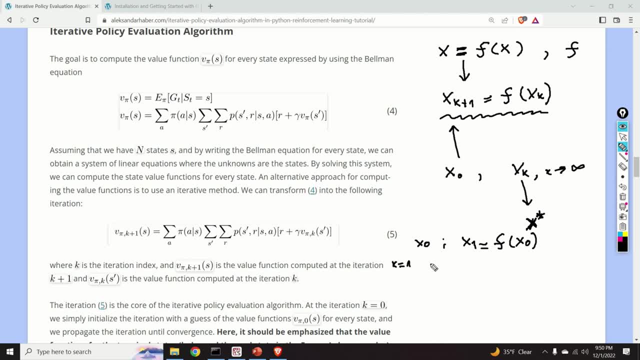 understand the cost of the iteration to find the correct answer for it. So we make the next step. k is equal to 1,. we have the following: We compute x2 as f of x1, where this x1 is the x1 computed from the previous iteration. And we continue this process, And for sufficiently. 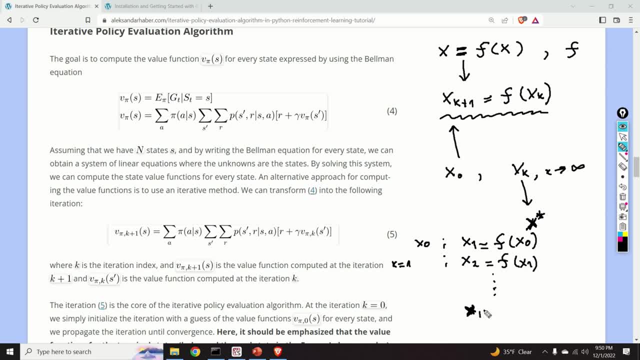 large k, our xk will converge to the true solution. Again, the convergence is not always guaranteed. It depends on the properties of this function f. However, in the case of the Bellman equation, we can use this iteration, that is, we can use the fixed point iteration. 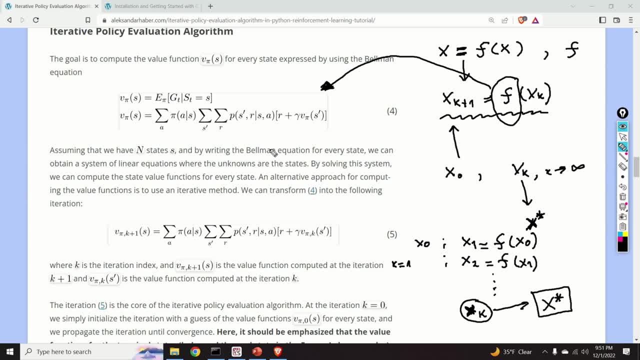 to convert the true solution And we can use this iteration to convert the true solution to the true solution. And we can use this iteration to convert the true solution to iteratively solve the Bellman equation, that is, to compute the value function. Okay, 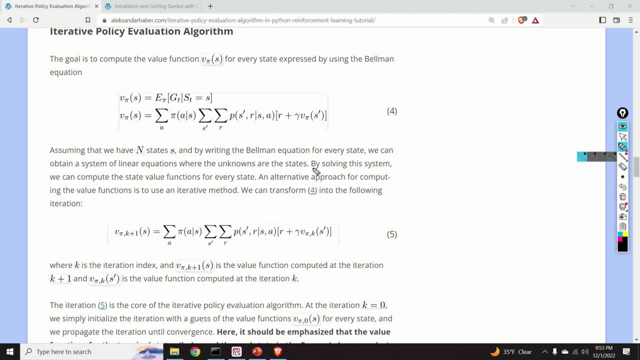 so let's use this trick to solve our Bellman equation. What is the main idea? The main idea is to transform the Bellman equation into an equation that's iterative, And here is the result. So what did we do over here? We simply included an index k over here and an index k plus 1. 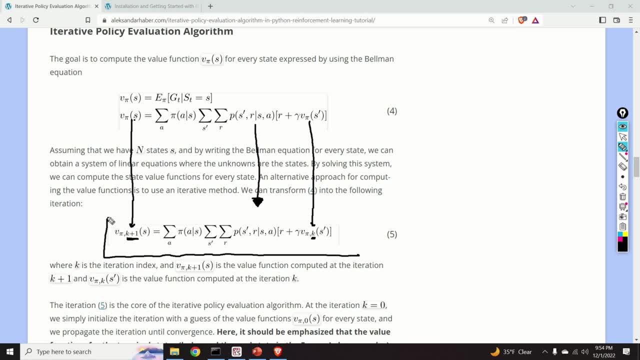 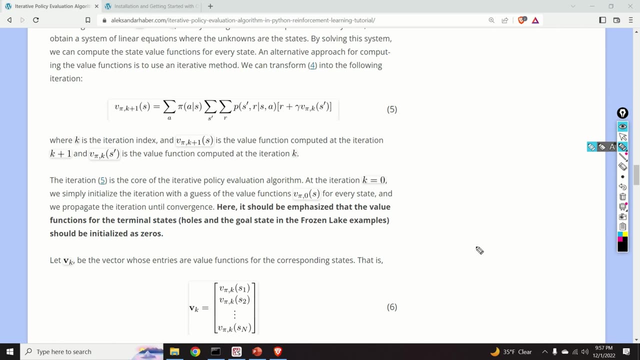 over here. And here is the iteration. And this equation is in the core of the iterative policy evaluation algorithm. At the iteration, k is equal to 0, we simply initialize the iteration, And here is the iteration. And here is the iteration. And here is the iteration. 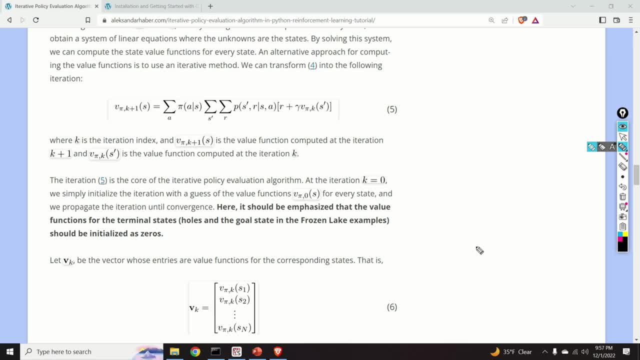 So we start with the iteration with a guess of the value functions And we guess the value function of every state, And then we simply propagate this iteration until convergence. Here it should be kept in mind that the value functions of the terminal states should be: 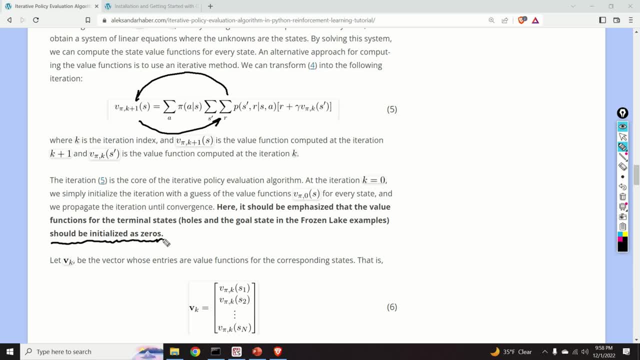 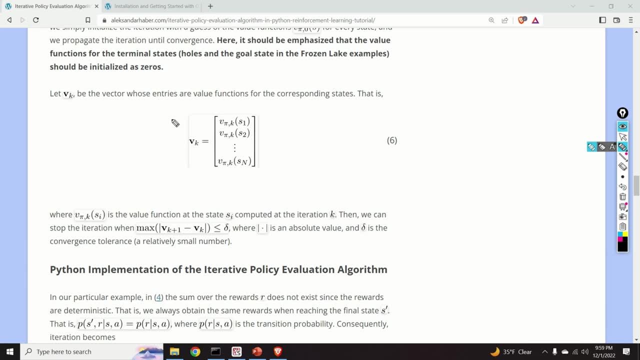 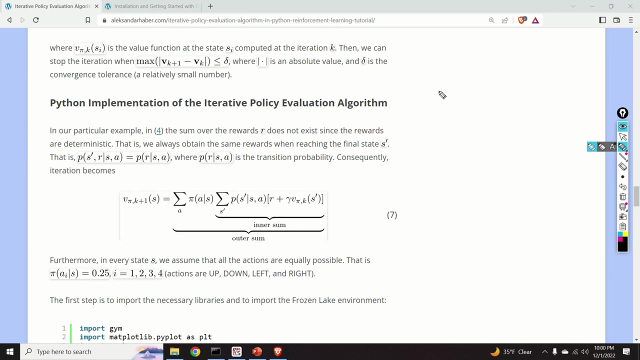 initialized as zeros, So keep in mind this fact. In order to implement this algorithm in Python, we group all the value functions, that is, the value functions of all the states, in the vector VK. okay, so what is the idea for implementing this algorithm in Python? well, we can split our iteration into two sums. be careful. 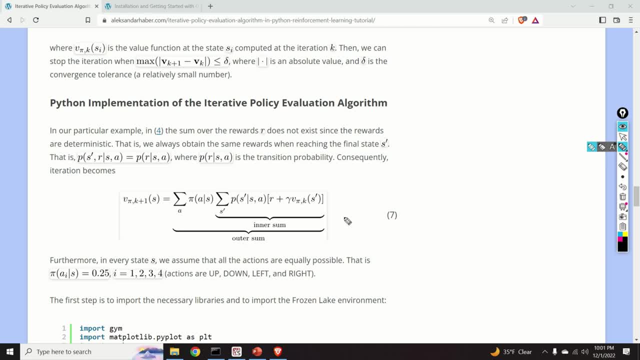 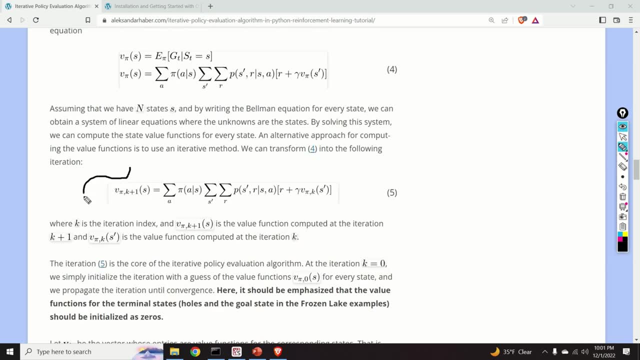 here. I said two sums. however, going back to the original form of our iteration, that is, by analyzing this equation over here, we can observe that we actually have three sums. we have the sum over a, sum over s prime and the sum over R. however, in the particular example that we are considering, that is in the case. 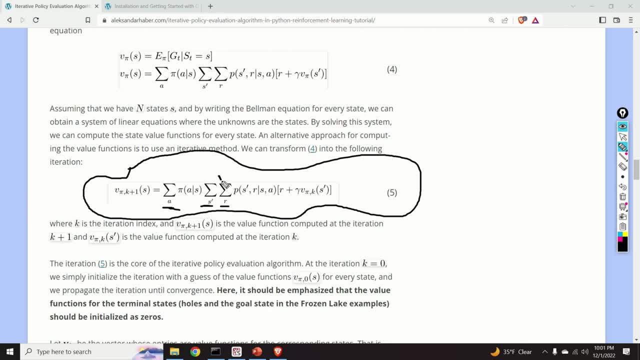 of the frozen lake example, the sum over R does not exist, since the dynamics, that is, this probability over here, does not include R, since we assume that the rewards are deterministic. so p s prime comma, R given s and a is equal to probability of s prime given s. 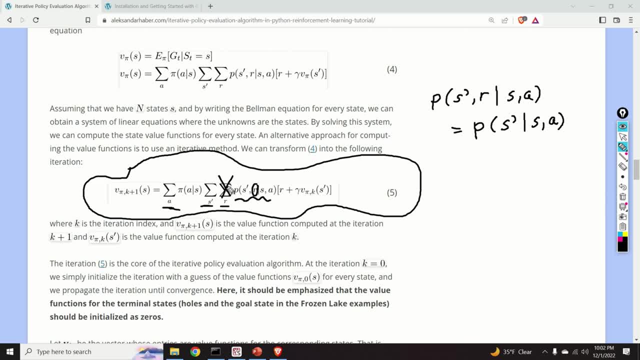 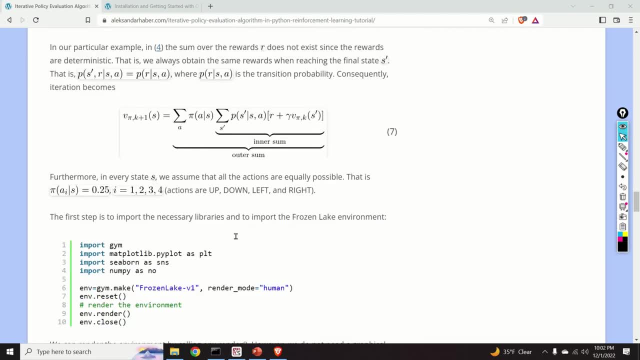 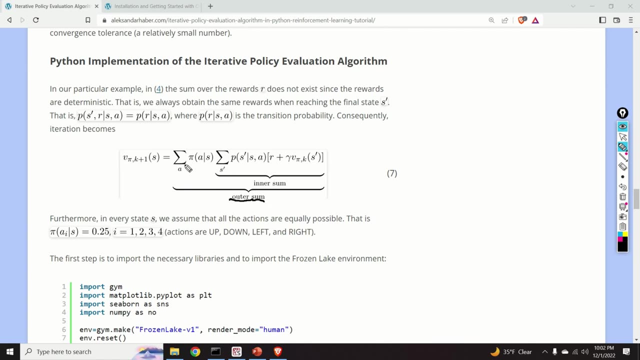 and a. consequently, we don't need to sum over R, and this fact significantly simplifies the implementation. consequently, over here we will have the outer sum and this sum will be performed over the actions, and then we have the inner sum that will be performed over the next states. here's the Python. 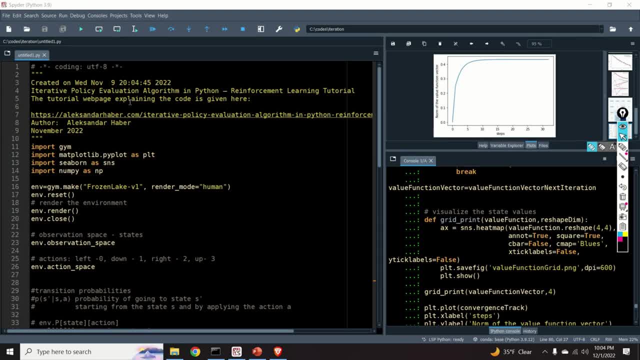 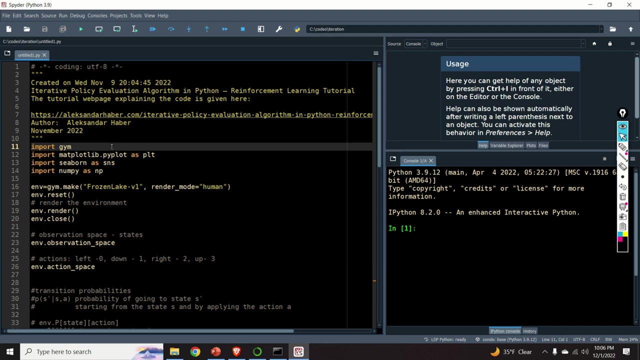 implementation of the iterative policy evaluation algorithm. as you can see, I'm using the spider environment in anaconda. I like spider very much sense. it reminds me of MATLAB. I can simply select certain code lines, I do the right click and I can execute these cold lines. as always, the first step is. 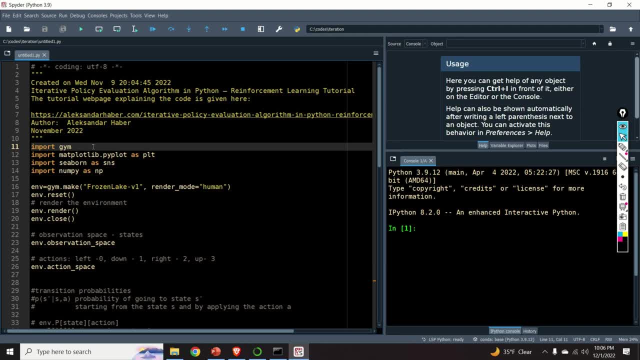 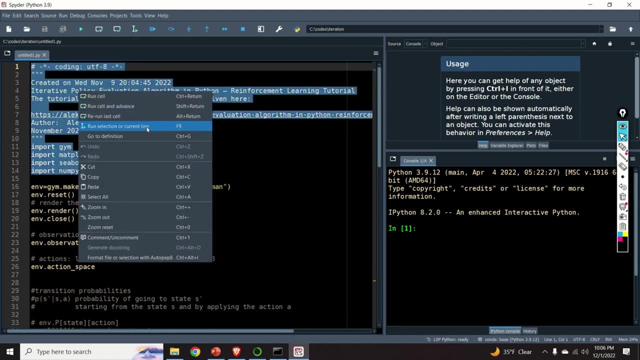 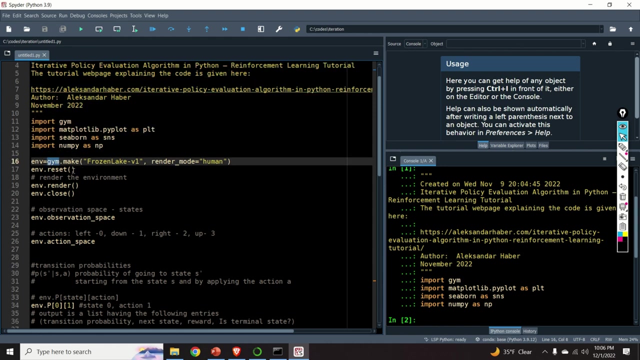 to import the necessary libraries. we import the gym library comment tree library5.ctp in this videoür. we import the plotting tools, then we import this nice library for plotting, seaborn, and finally we import the numpy. so let us import the libraries. next, let us create our environment. we call the function gym make. we specify the name of the. 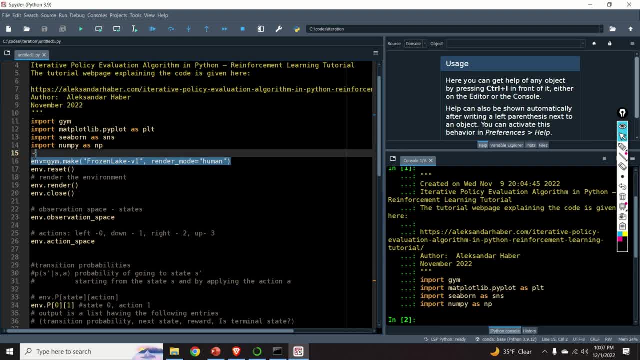 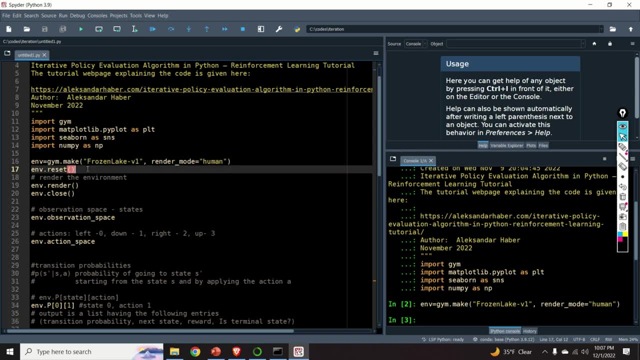 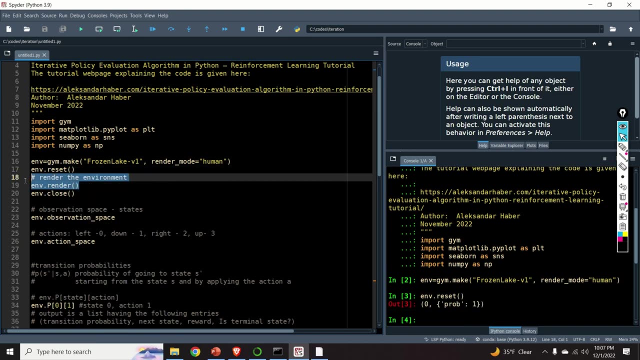 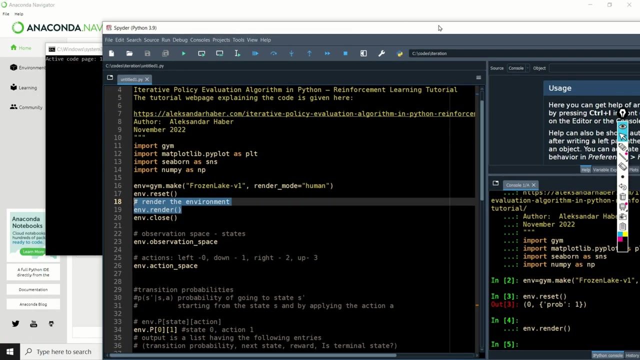 environment and we specify the render mode. let's do that. nothing happens, of course. nothing happens because we have to reset the environment. then we need to render the environment in order to visualize our problem and let us find the rendered environment. here is the rendered environment it has. 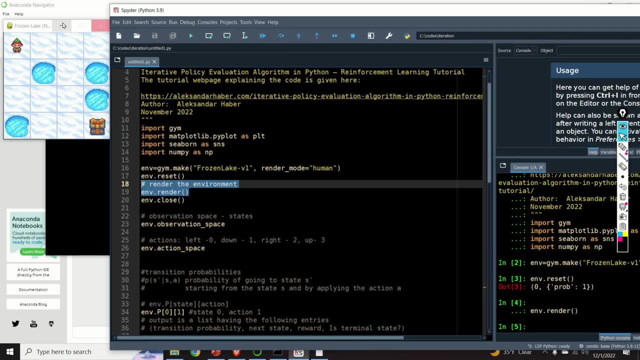 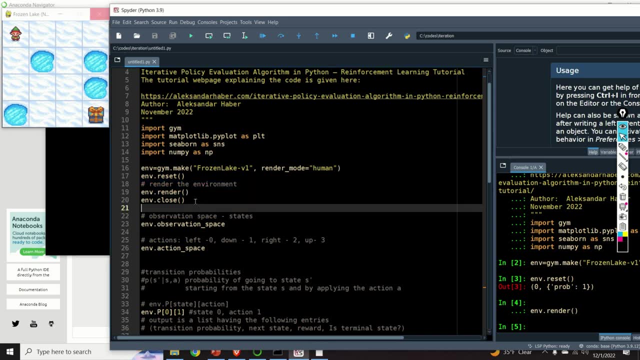 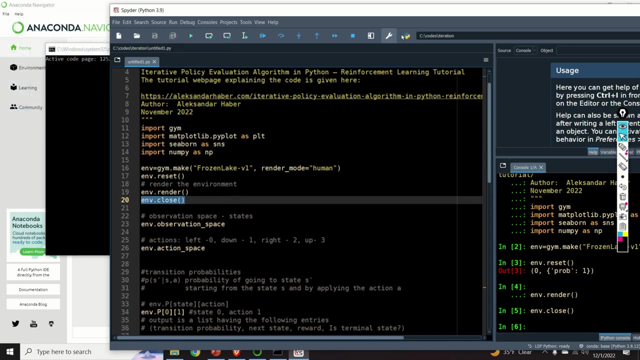 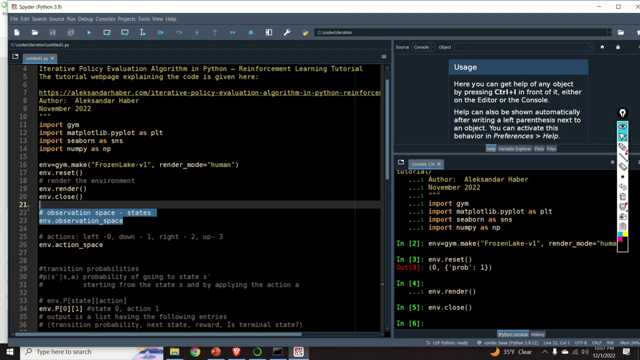 to be rendered in order to visualize our problem. and let us find the rendered environment in order to visualize our problem, and let us find the rendered environment. consequently, we can simply close the gui, that is, we can close the graphical representation of our environment. okay, let us look into the observation space, that is, let us check the number of states. 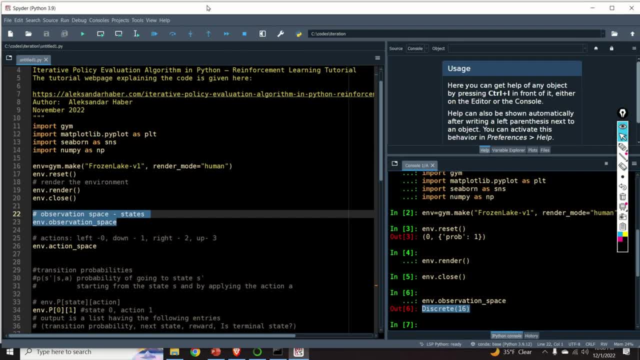 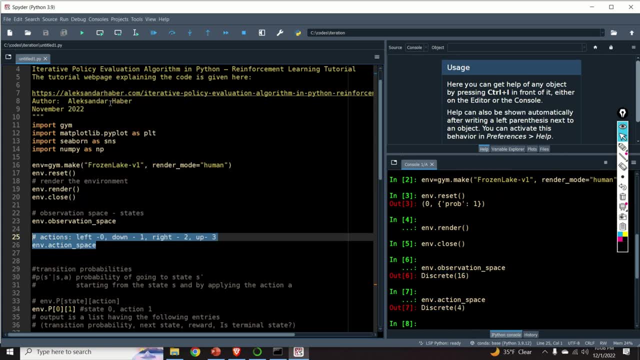 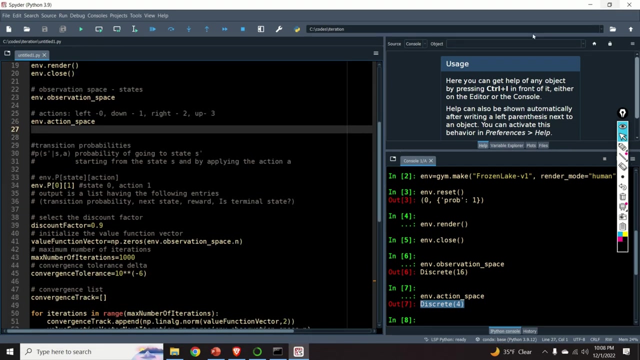 good, we have 16 states. that's what we expected. then let us check the action space. uh-huh, we have four actions. these actions are up down left and right. good, everything is as we expected. the next step is to inspect the transition probabilities. so let's go back to our post and let 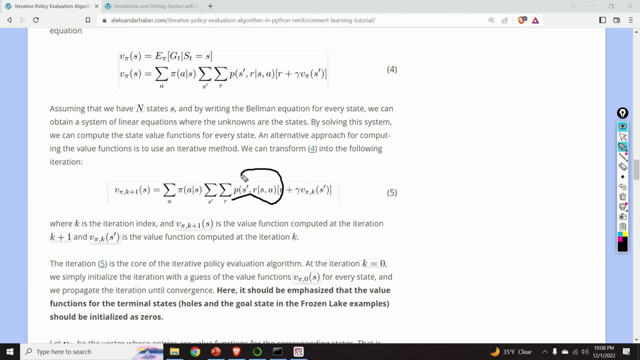 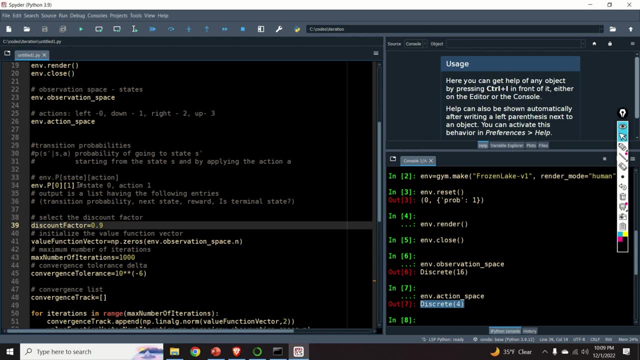 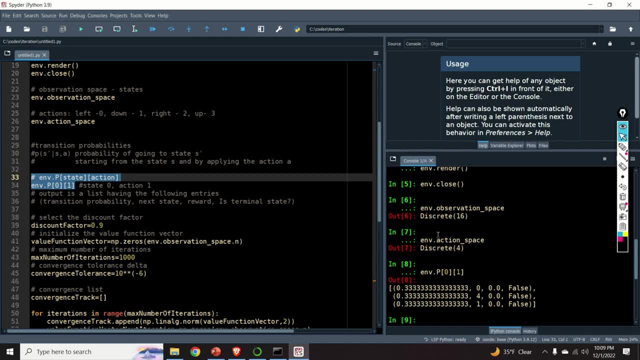 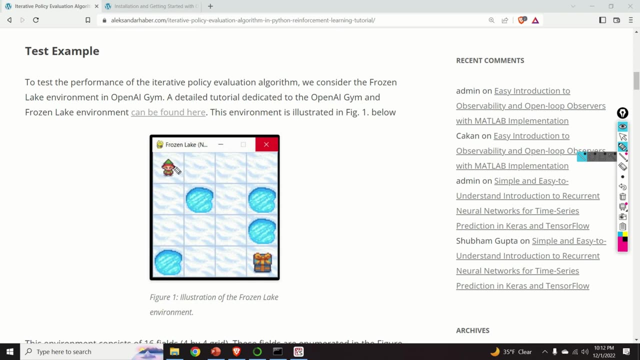 to provide me the dynamics, or better to say, the transition probabilities, of being in state zero and selecting the action one. by typing this code line, we asked the open aigim: what is the transition probability of being in this state? and by applying the action down, let us analyze the result. 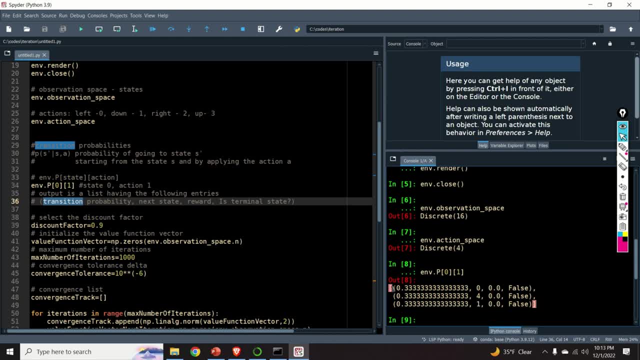 here is the result: we obtain a list with three elements. the entries in every element should be interpreted as follows: this part over here is our transition probability, this part over here is the next state, this part over here is the reward and this false over here is actually a boolean variable. that 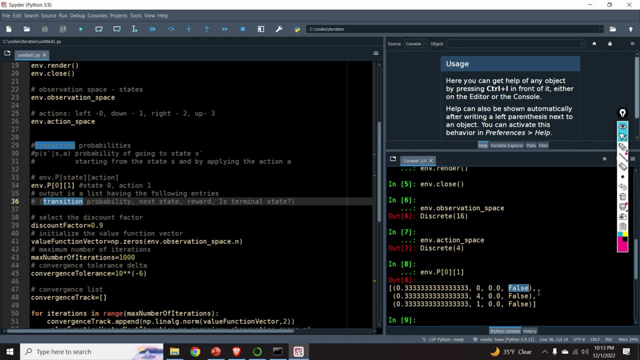 provides us an answer to the question: is the next state terminal state? in this case, the next state is zero, and this is obviously not a terminal state. so the interpretation is the following one: we are currently in the state zero, so we type p and we have zero over here. 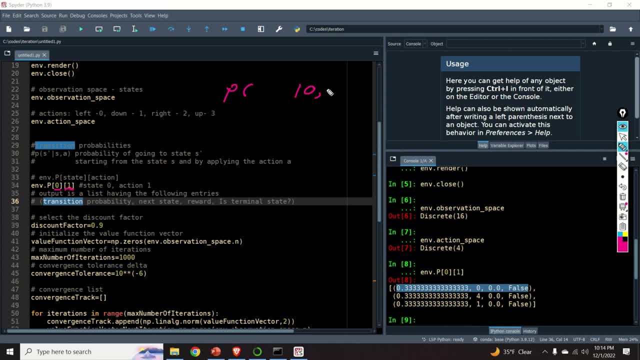 this number number over here. one is the applied action. the applied action is going down. the next state is given over here is zero, and this number over here is the transition probability. so this probability is equal to 0.33 and three, three repeats itself, so there is a chance of one over three off. 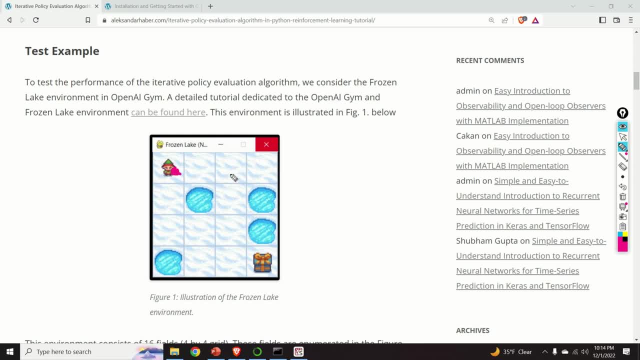 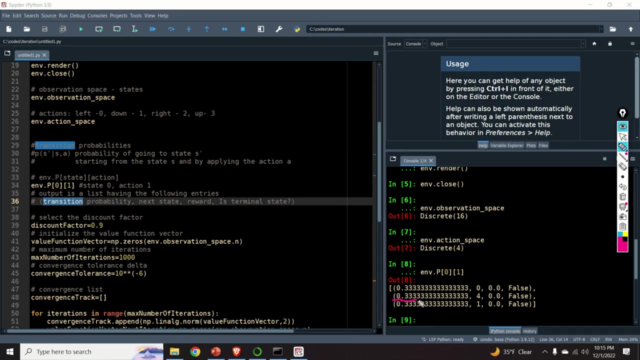 staying in the state zero. if we were in the state zero and if we applied the action down again, there is a probability of one over three off staying in state s zero. if we were in the state s zero and if we applied the action down. let us analyze this transition probability. 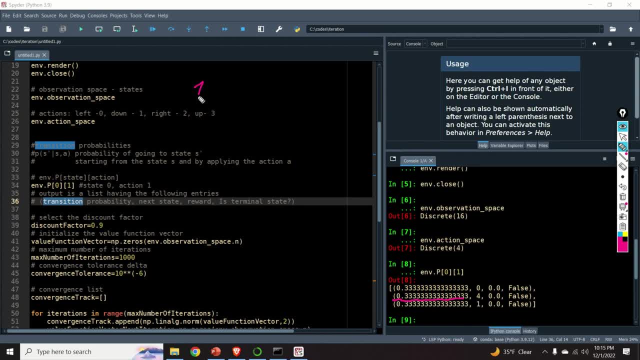 so what's happening over here? again, we have probability, the current state is zero, the action is one, which means down, and the next state is the state four, as we can see over here, and the transition probability again is one over three. okay, so let us go back to our graphical representation and let us represent. 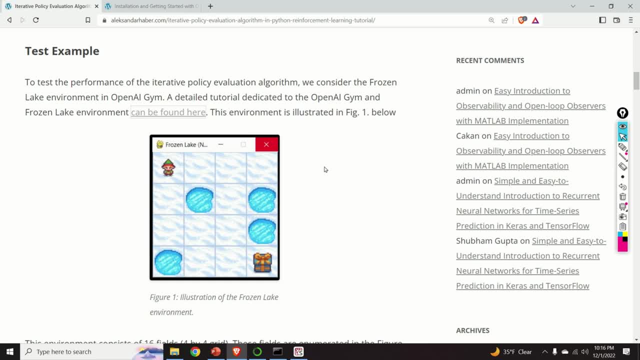 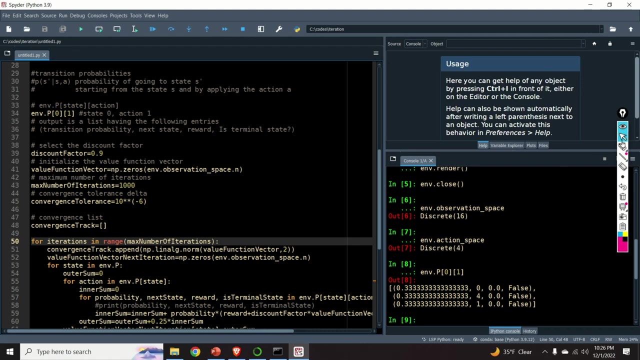 this graphically, so there is a probability of one over three off going to this state. the state is the state four if we were in the state 0 and if we applied the action go down. now that we verify the transition probabilities, we can proceed with the implementation of our algorithm. 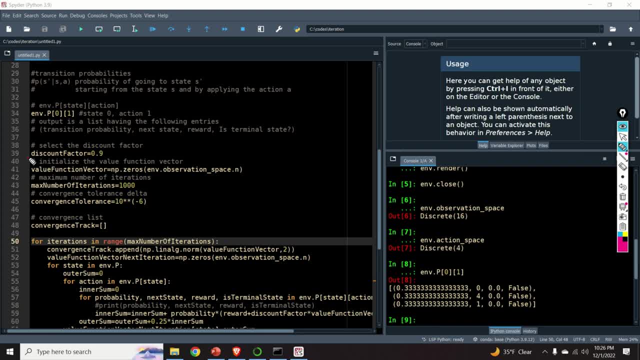 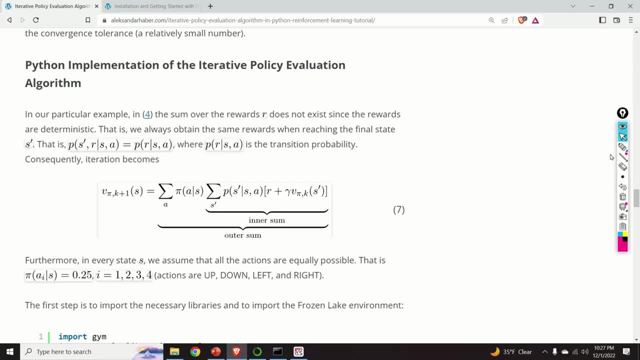 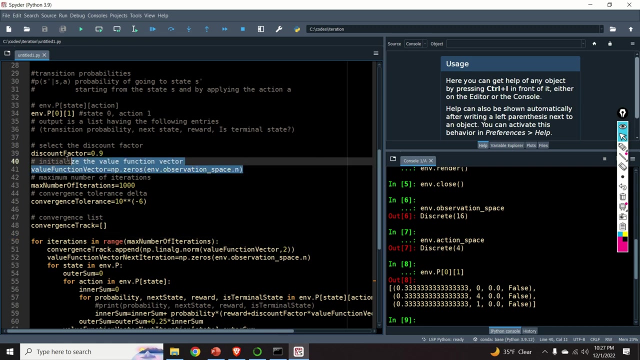 the first step is to prosecut this algorithm, select the discount factor, and the discount factor is this number over here it's the number gamma. usually we select this number in the interval from 0 to 1- in my case, I selected gamma to be 0.9. then we initialize the vector storing. 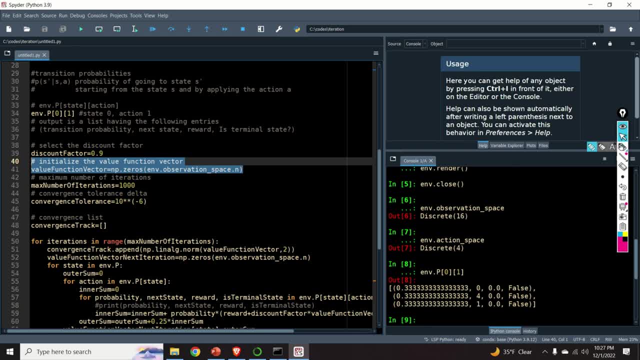 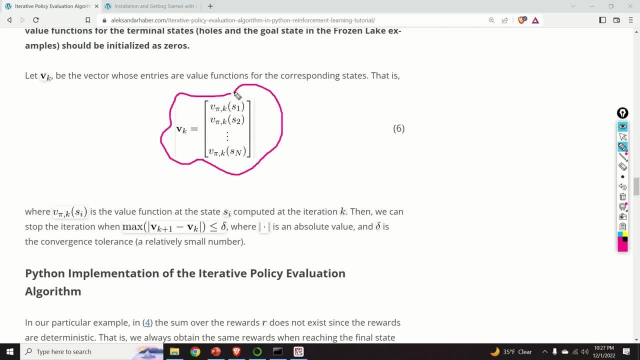 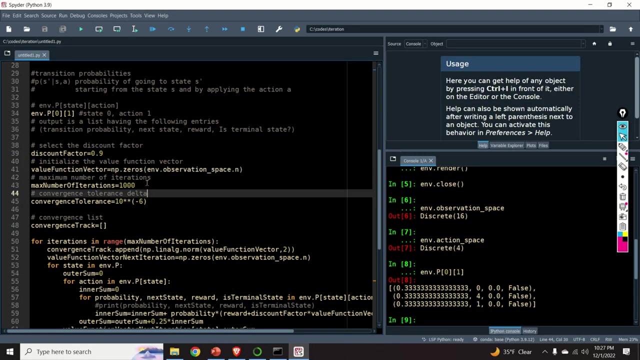 value functions for every state, that is, we initialize this vector over here. we select every entry of this vector as 0, so every entry is equal to 0. then we select the maximum number of iterations- K- in my case it's 1000. Then we select the convergence tolerance: delta. 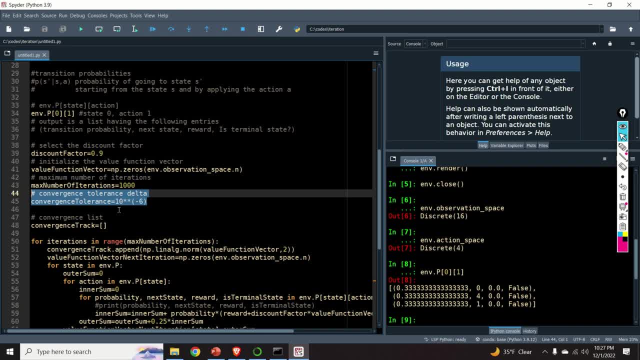 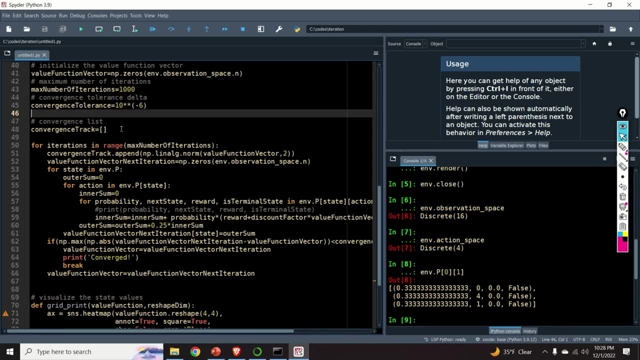 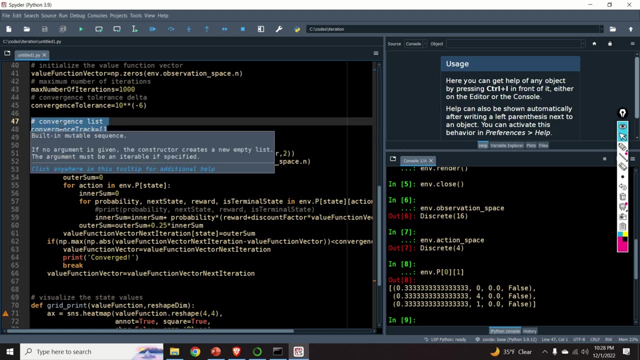 The convergence tolerance delta is 10 to the minus 6.. As you will see later on, the algorithm converges quite quickly. Next, we initialize a list that will track the convergence of the algorithm. This list will be used for visualization purposes, as you will see later on. 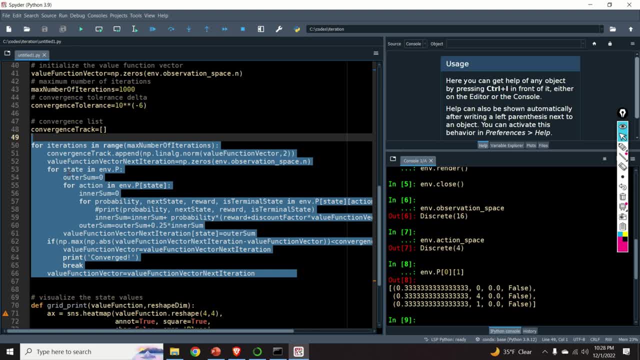 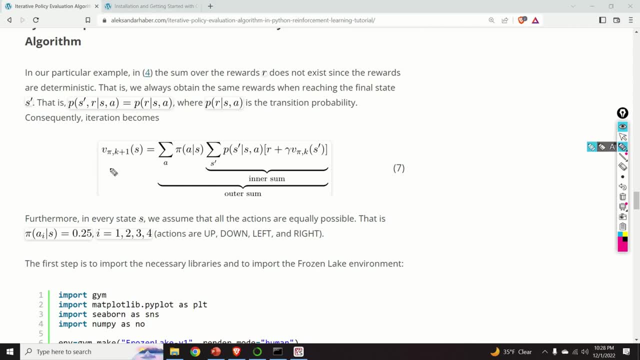 This part over here implements our iteration. Let's go back to our iteration once more. What do we have over here? Obviously, we need to iterate over k. Then, for every fixed k, we need to compute the outer sum. And to compute the outer sum, we need to have a for loop that will go over the actions a. 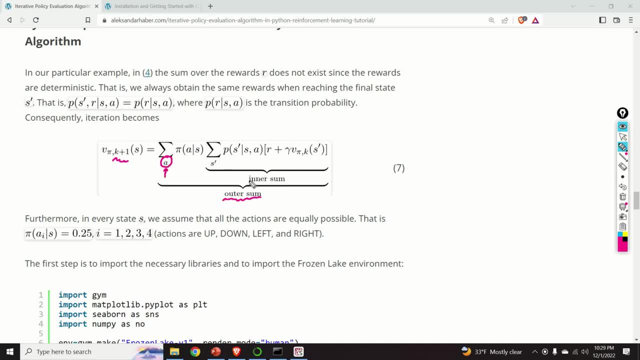 Then for fixed k, we need to compute the outer sum. Then for fixed k, we need to compute the outer sum. Then for fixed k, we need to have another for loop that will evaluate the inner sum, And this for loop will iterate over s prime. 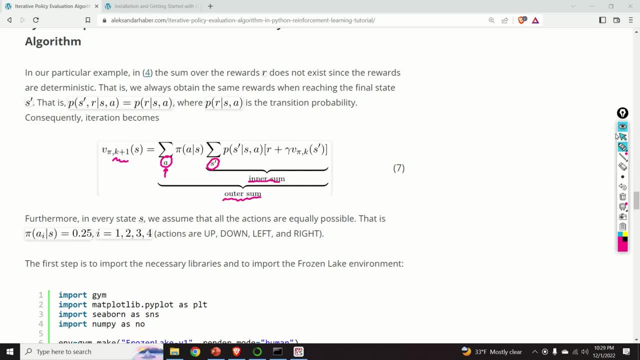 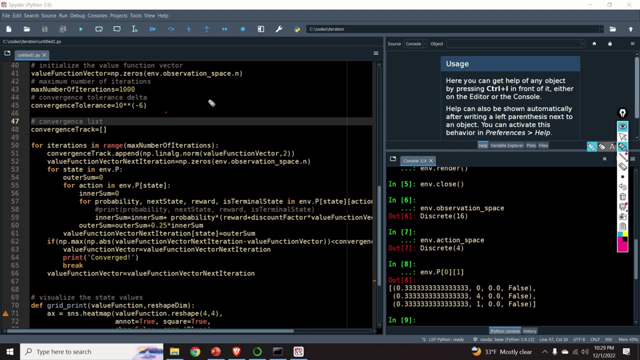 That is, it will iterate over the next states. Okay, so here is again our code. This for loop over here iterates over k, That is, it will compute. Okay, So we have k plus 1, the vector containing value functions for the next iteration. 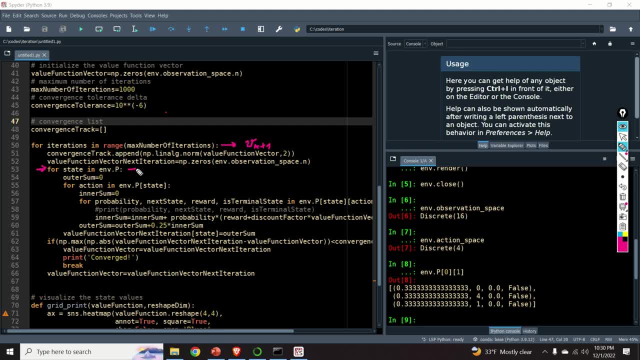 This for loop iterates over the states in our environment. In our case, this state variable goes from 0 and it ends at 15.. Then we need to compute the outer sum. Okay, So we have to compute for the next iteration. 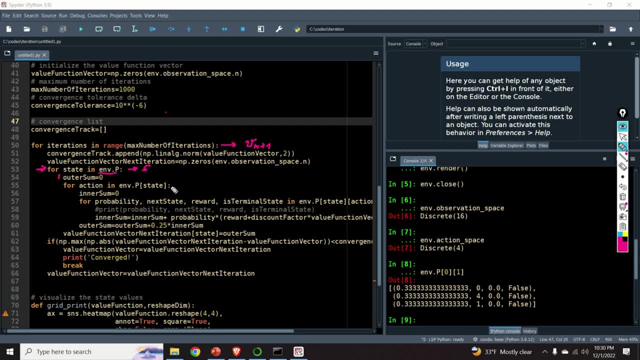 And also here this will be a remember- function of z. And then we need to compute the outer sum. To compute the outer sum, we need to iterate over the actions, So this for loop iterates over the actions. And finally, we need to compute an inner sum. 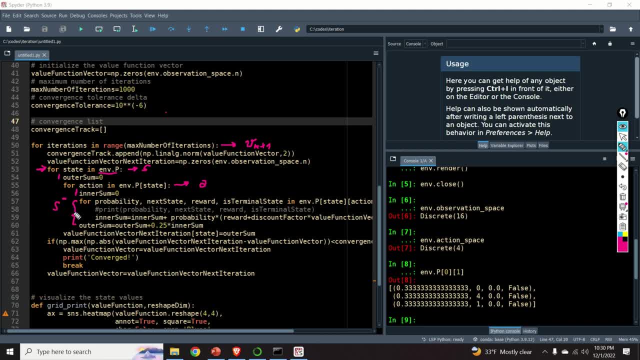 That is, we need to iterate over the next states, And this for loop iterates over the next states S prime And it computes the inner sum. Alright, Any question, Please? We are now Star Ting sum. Finally, over here. we test the. 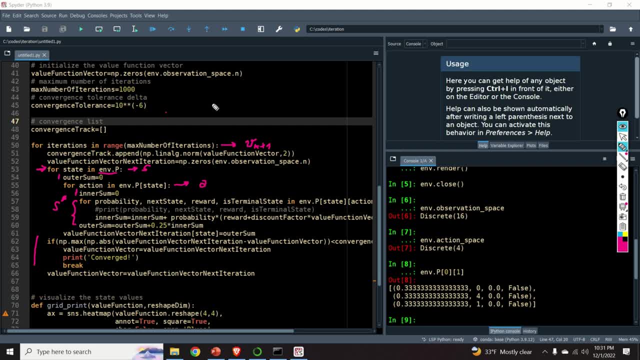 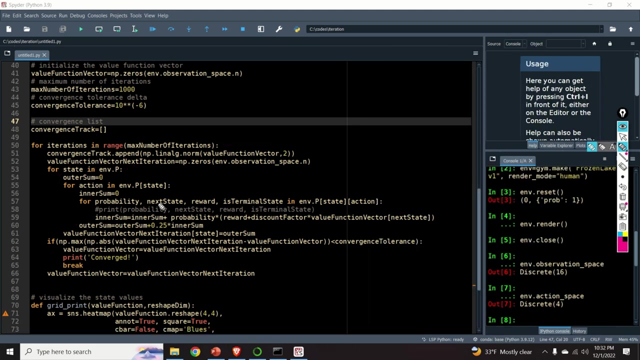 convergence. If the difference between basically vk plus 1 minus vk is small enough, we stop the convergence. That is, if this difference is below the convergence tolerance, we stop the algorithm. Here are a few important comments related to this algorithm. Let us first focus on this part over here. 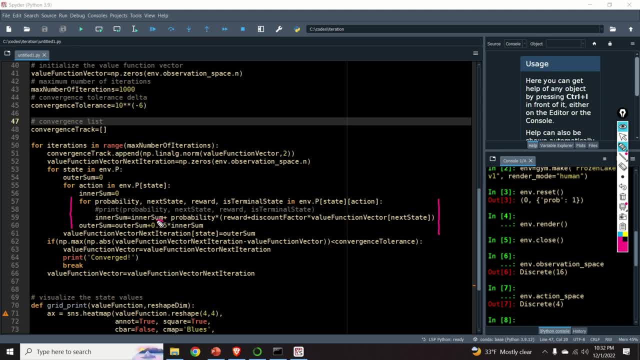 This part is my probability of selecting a certain action. In my case, I'm assuming that all four actions are equally possible. That's why you have here 0.25.. Now let's look at the probability of this part over here. computes the inner. 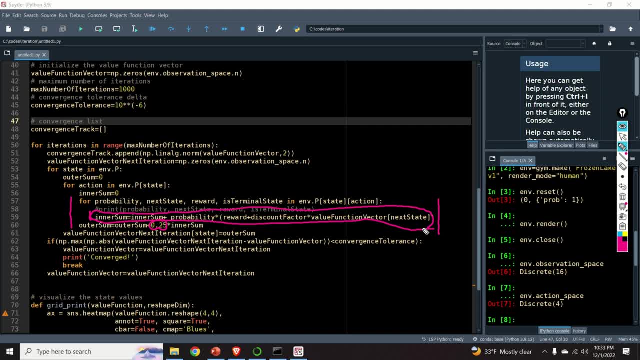 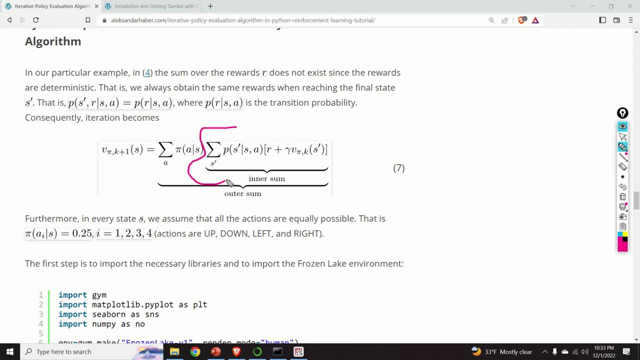 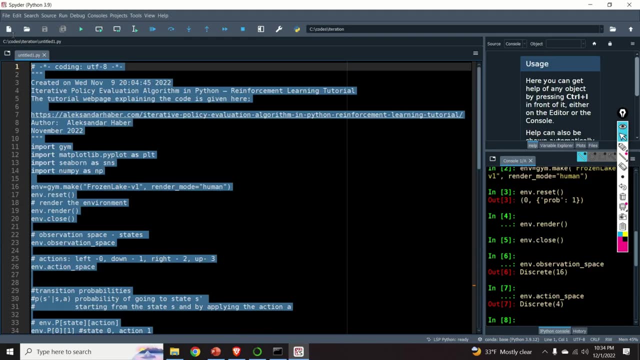 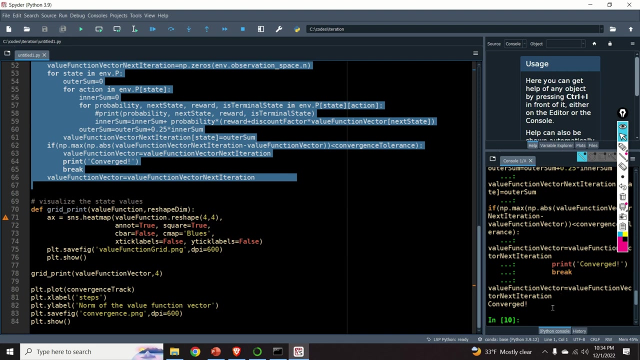 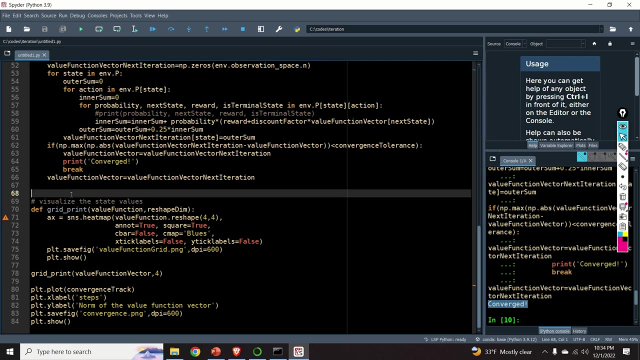 sum and again the inner sum is defined over here. Now you're ready to run the algorithm. I will simply select this part, do the right-click and converged. I obtain the message that my algorithm converged, So let us visualize the results. I defined this. 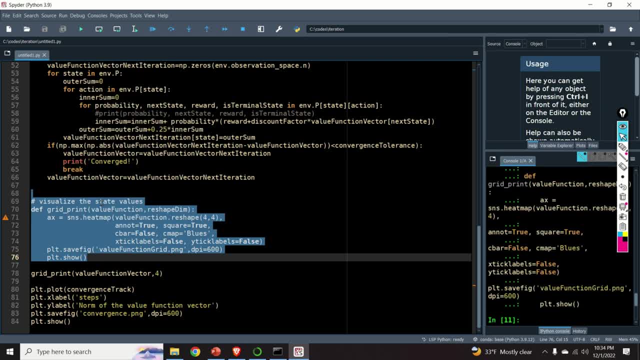 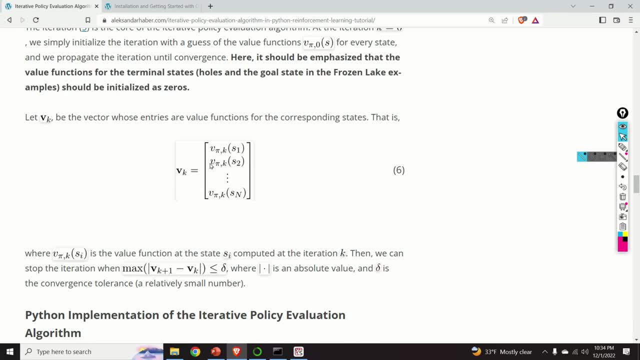 function over here to visualize the results. Basically, this function will take my vector vk and it will transform this vector into 4x4 grid and do a plot, or do better to say, a, a heat map that will visualize the values of the value functions. 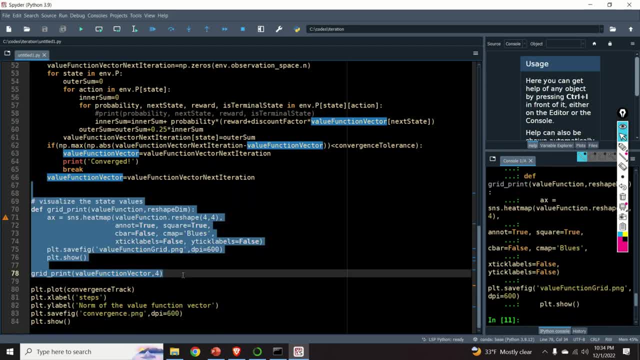 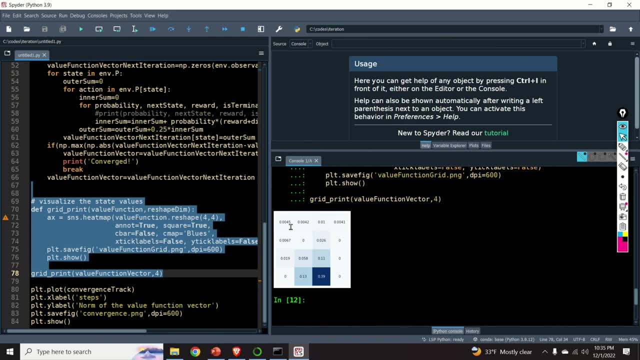 So let us see the result. Here it is. Here are my value functions. This is the value function for the state S1.. This is the value function for the state 1,, 2,, 3,, 4,, 5,, 6,, 7.. 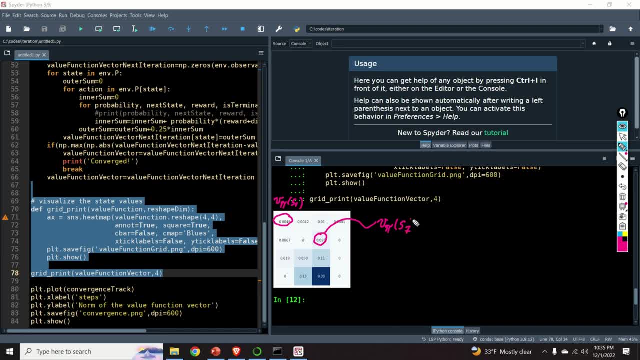 So this is V, pi, S7. And here you can observe that the value functions for the terminal states are zeros. That is a good check that can verify the accuracy of your implementation. Consequently, we have accurately implemented The algorithm, since we can see over here that the value functions in terminal states. 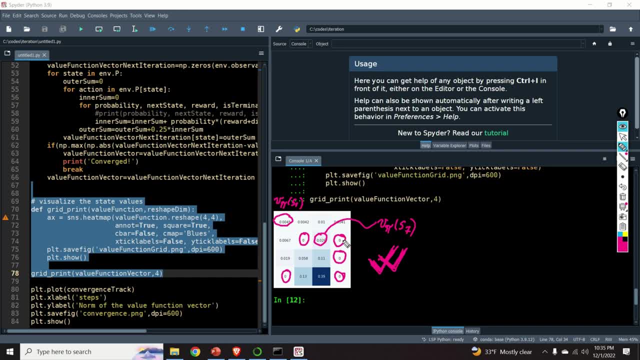 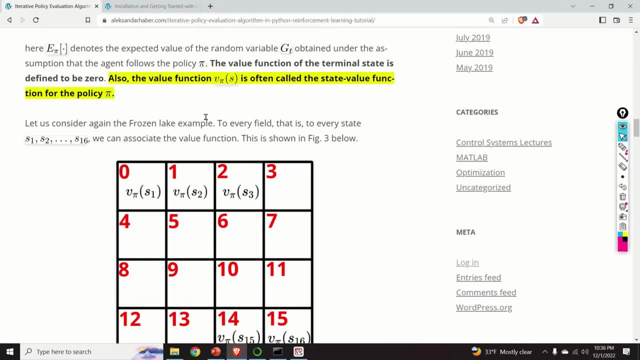 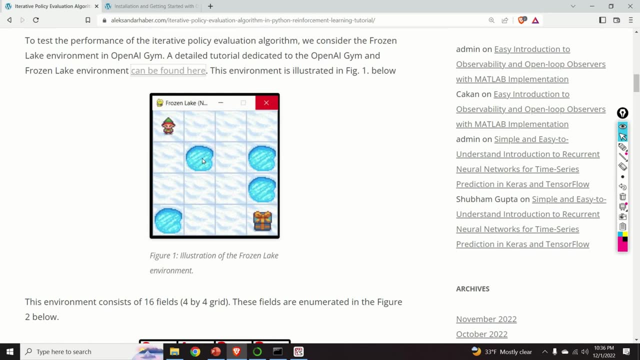 are zero And you can simply verify that these states are actually terminal states by going back to our graphical representation and by looking at the structure of the frozen fields and the whole fields. Obviously, here we have a terminal state, here we have a terminal state, and these three 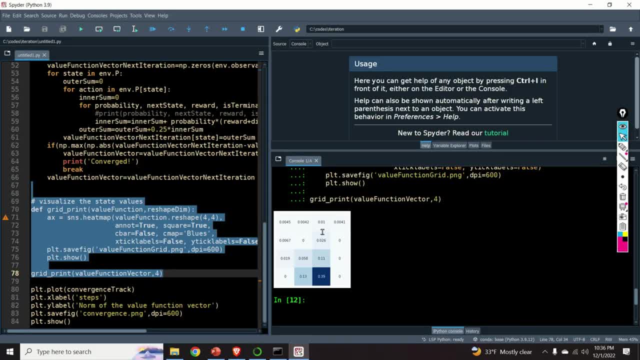 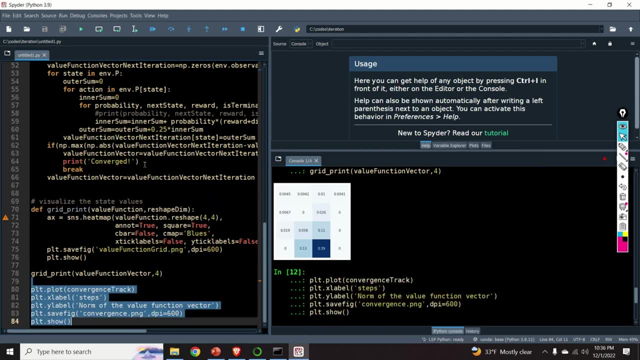 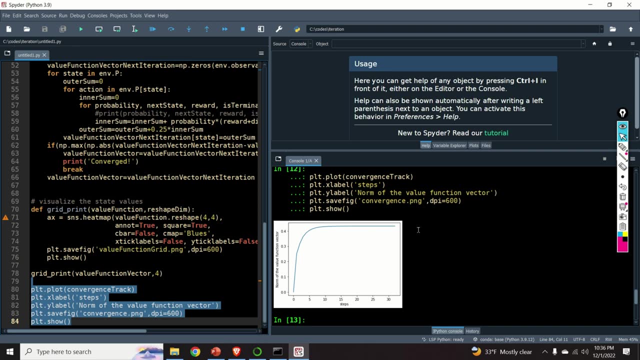 states are the terminal states. So the way you can look at this graph is that these particular sets under these determinations, are the torment states, as 3 forms of state 2 and 3.. So again, there are major farmingusstates and this corresponds to our results. 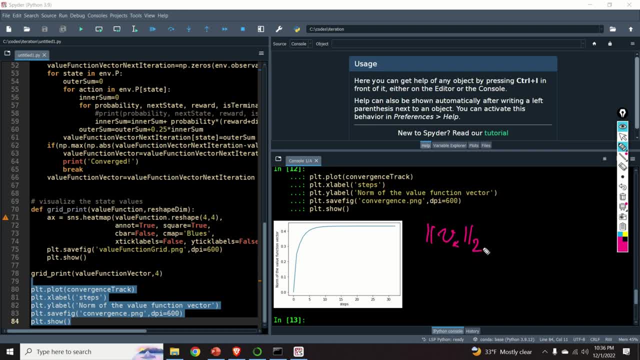 And finally, let us plot the convergence. Basically, this graph plots the 2 norm of the vector vk. six or seven iterations. our algorithm converges. okay, that would be all for today. i hope that you like this video. if you like the videos i create, please. 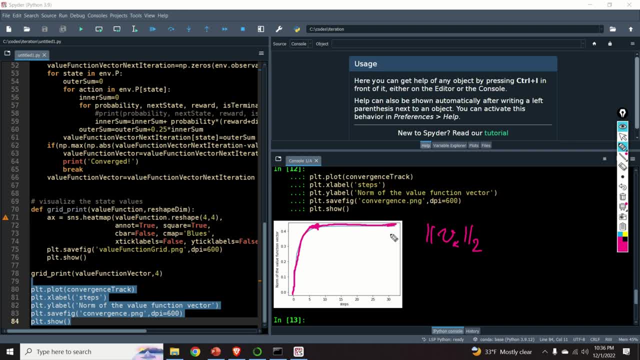 press the like and subscribe buttons. thank you very much and have a nice day.